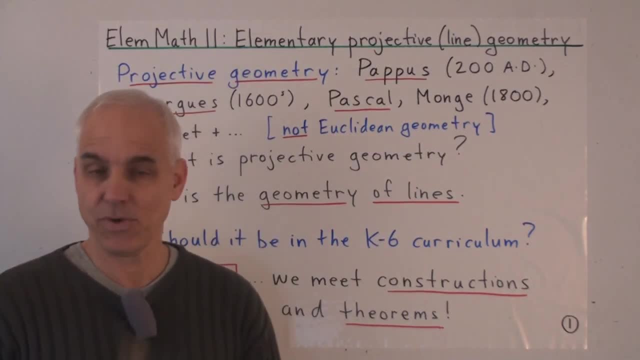 In fact, it's more elementary than Euclidean geometry. So we are not doing standard Euclidean geometry, We're doing something which properly precedes Euclidean geometry. So what is this projective geometry? Well, a simple kind of definition is that it's the geometry of lines. 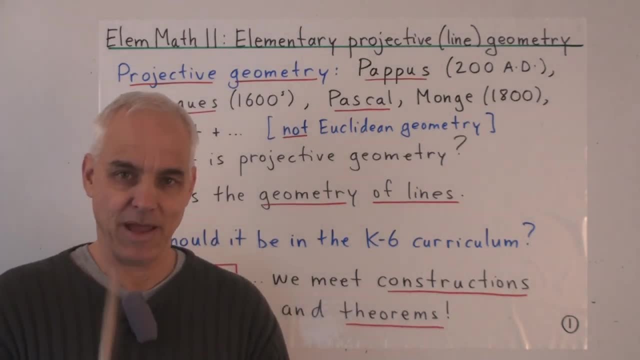 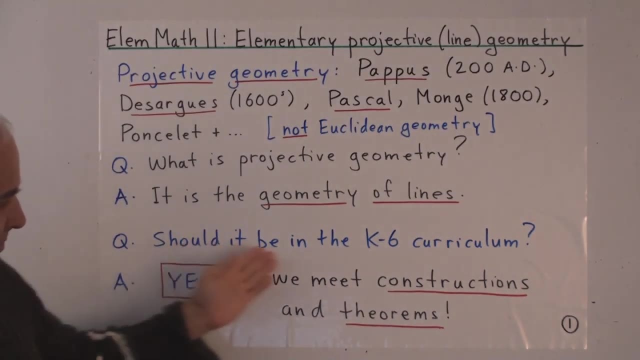 It's what we get when we look at the world just with a pen and a paper and a straight edge. Should this subject be in the K6 curriculum? I most definitely think the answer is yes. This is an excellent subject for young people to learn about, first of all, basic geometrical constructions. 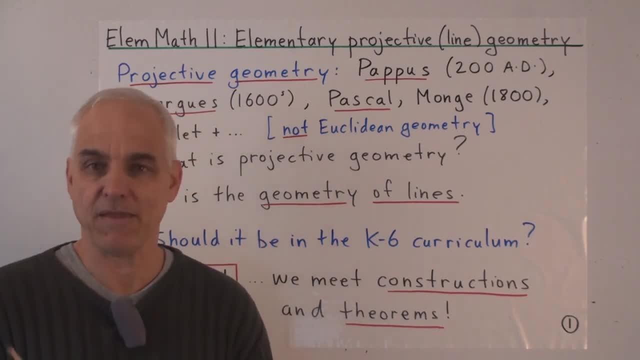 And also to meet for the first time the idea of a theorem. A theorem is a very important notion in mathematics, And what it is is a key result. A key result which is not obvious. Mathematics is full of theorems. 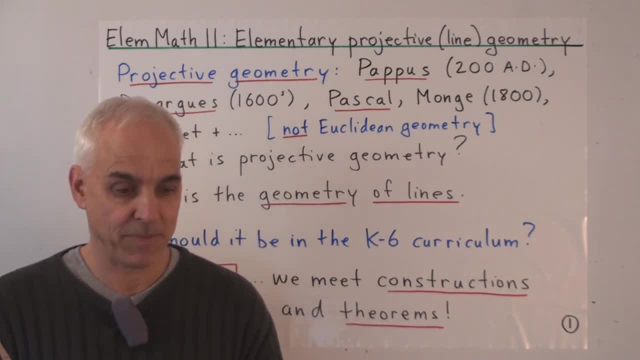 But many young students do not get exposed to them. They get more exposed to memorizing lots of definitions And learning algorithms for doing things. Those are all well and good, But mathematics has another side: The fact that there are these key results. 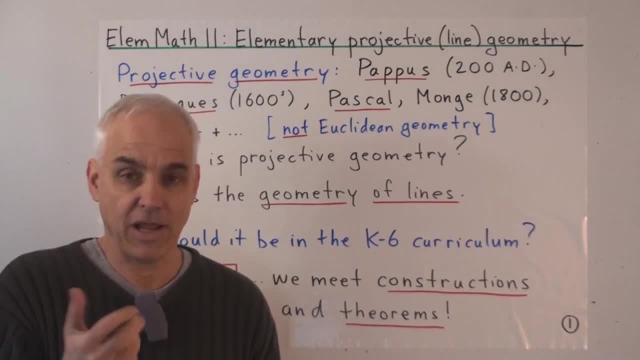 These key facts that are like jewels or like gems. We call them theorems, And in projective geometry even a very young student can meet some beautiful theorems, And you're going to meet a few of them today. So today we're just going to start with a gentle introduction to projective geometry. 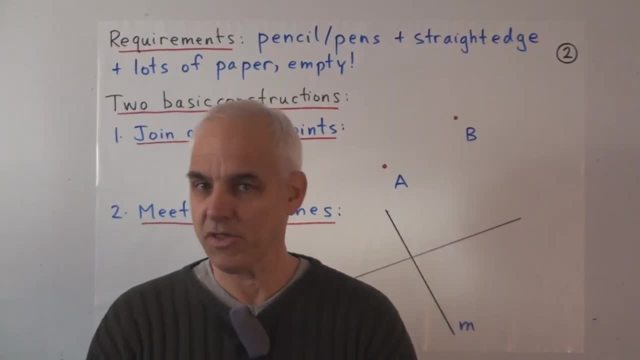 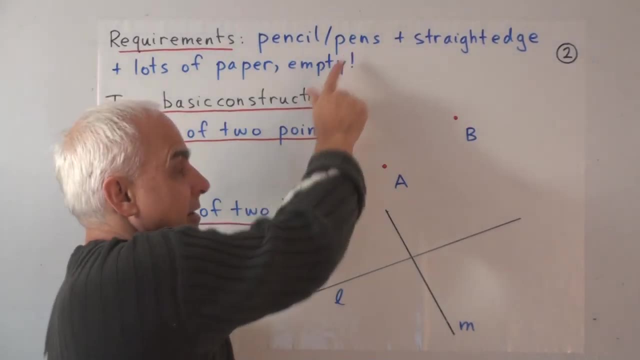 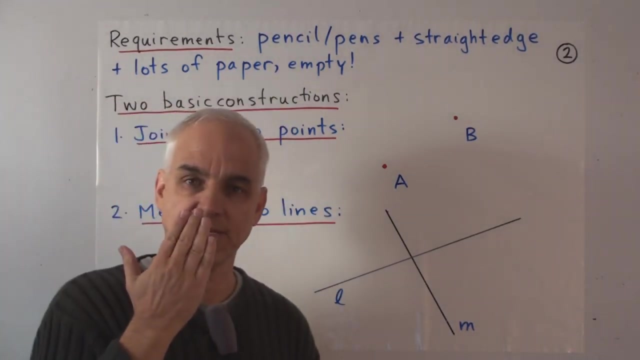 The geometry of lines. So what are the requirements that you're going to have to have to study this geometry? Well, we're going to need pencil or pens And we're going to need lots of paper, And the paper that we're going to use is empty paper. 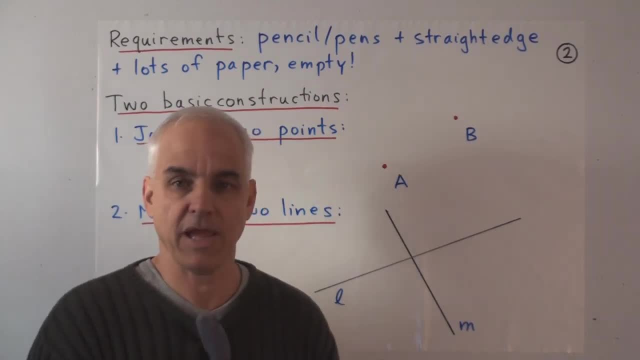 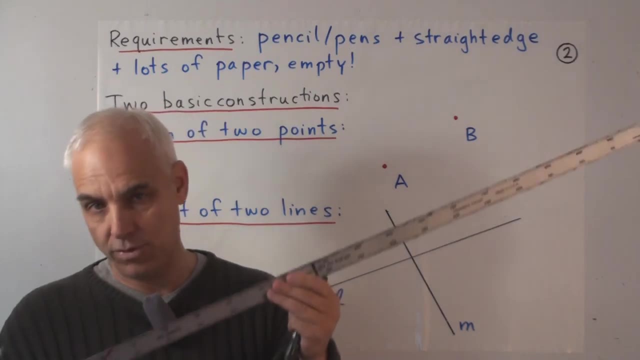 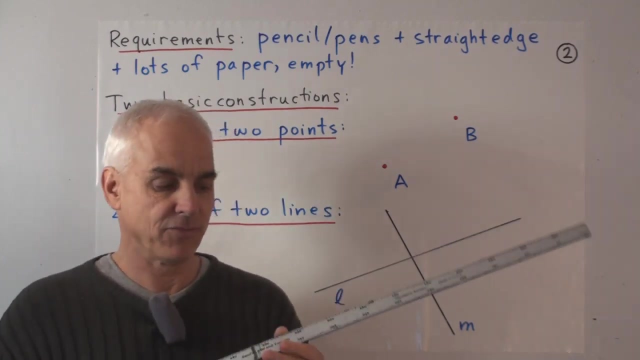 So not with grid lines, just a spare empty piece of paper. And we're going to need one more thing: A straight edge Or a ruler. But we say straight edge instead of ruler, because the actual ruler, because the actual marks on this ruler. 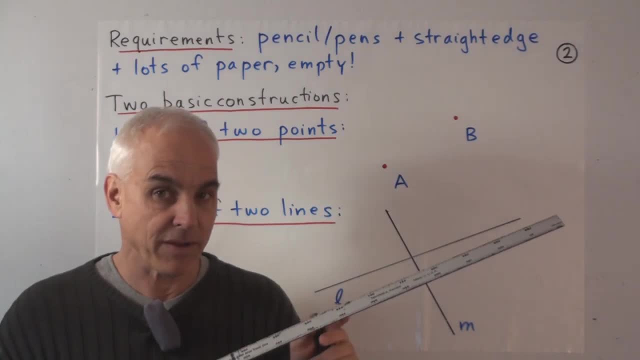 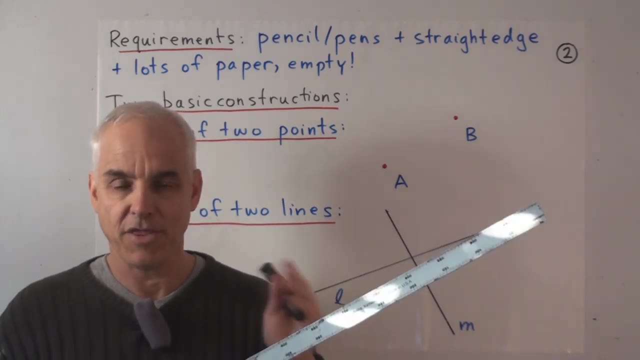 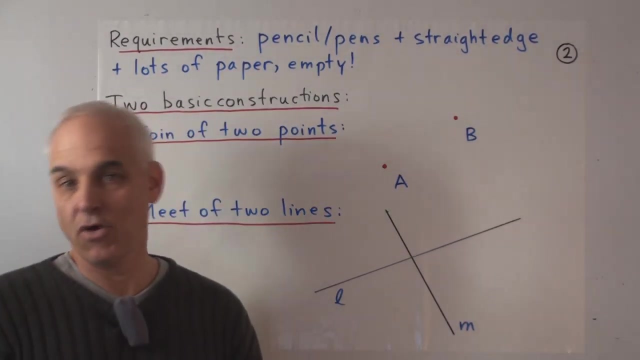 are going to be irrelevant for us. We're not going to be doing any measuring, We're only going to use this ruler to draw straight lines on the page, And there are two basic constructions that we use over and over again. The first construction is the join of two points. 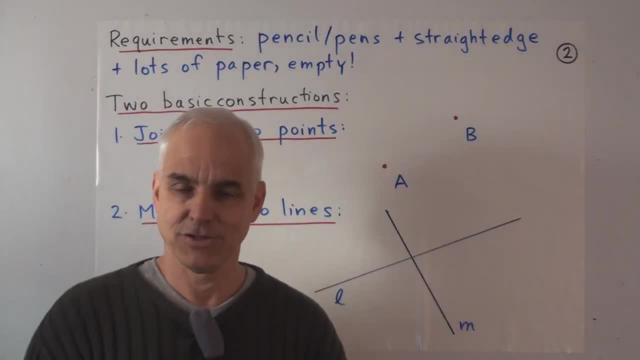 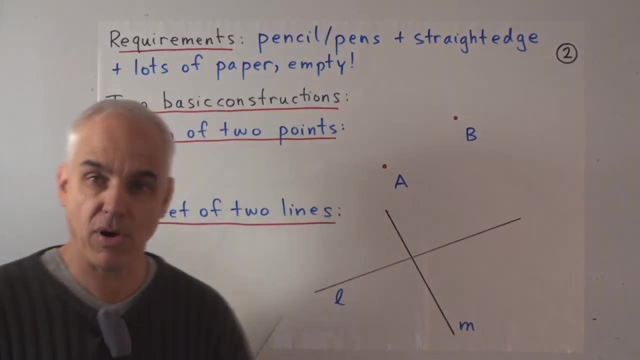 And the second is the meet of two lines. So let's illustrate these. So here are two points, A and B, And they're just random points on the plane. Given two random points, we can construct their join. The join of two points is a line. 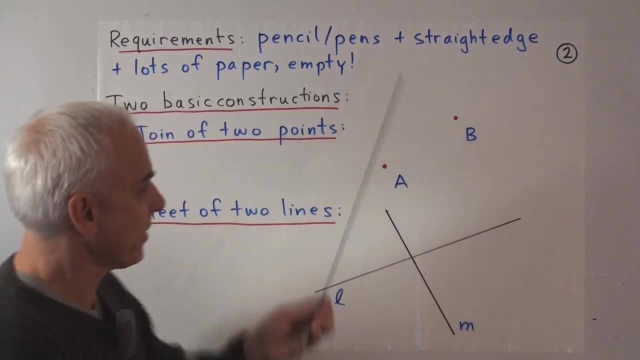 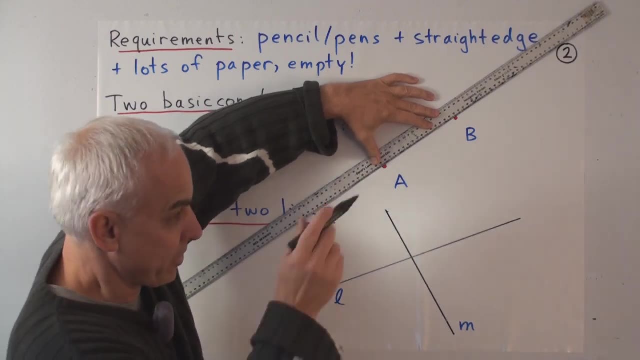 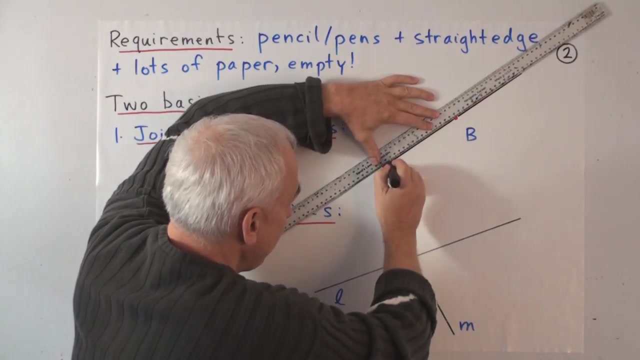 What we do is we take our straight edge and we put it down on the paper so that it's connecting the two points, And then we're going to join those two points with a line, And the line that we're going to draw doesn't have to start at A and B. 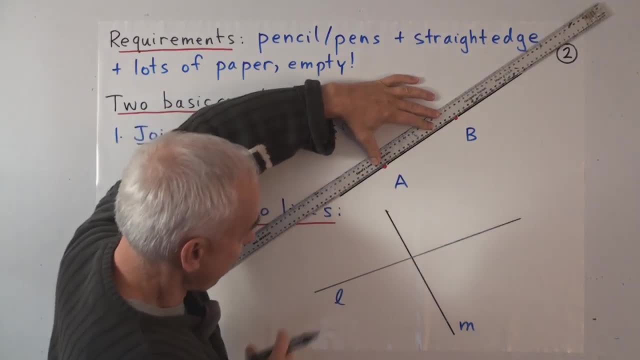 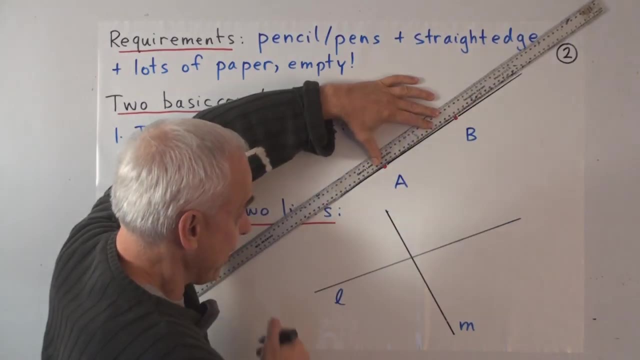 It just has to go through A and B Alright. so this is an important skill: to be able to put the ruler down, To hold it there firmly enough so that you can draw that edge without the ruler wobbling, And so that you actually do get a line through the two points. 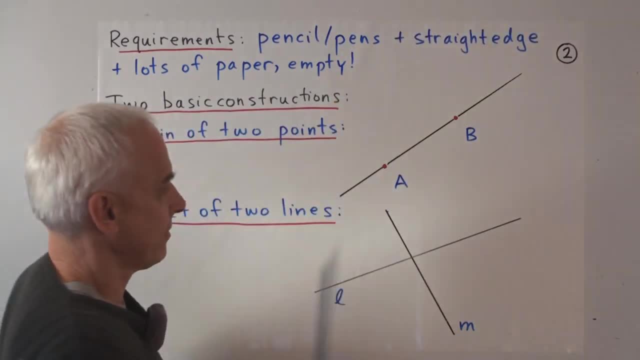 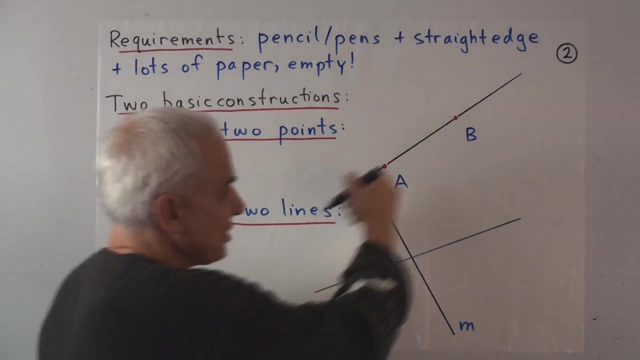 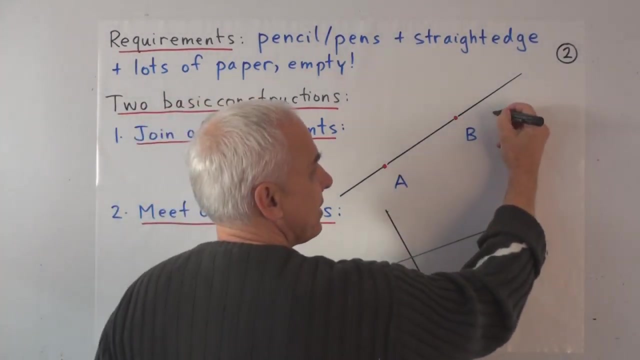 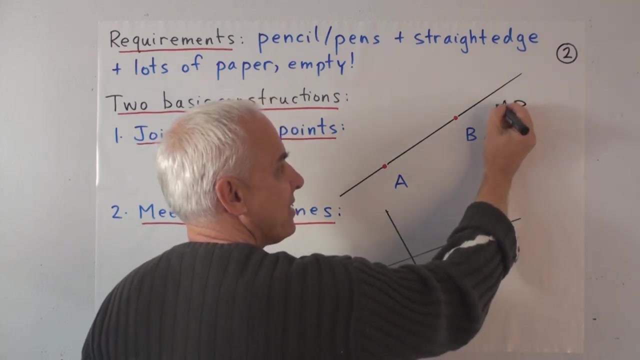 Not on one side or on the other. So that's a very physical skill that a young person learns. And we're going to give this line a name, Because it's the line through A and B. we might call it AB. That's the name of that line. 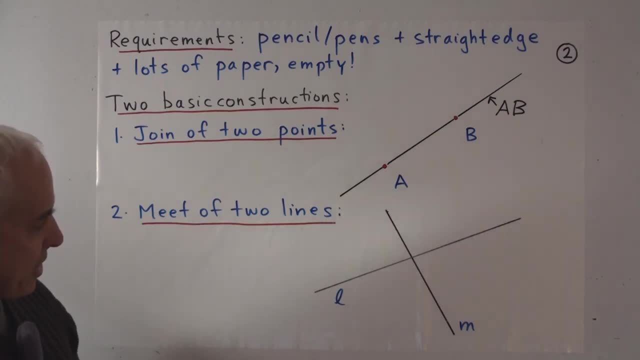 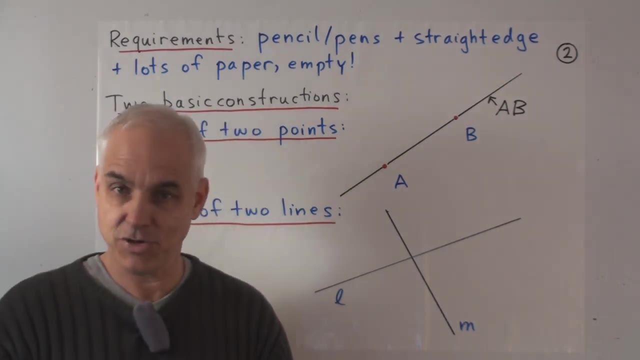 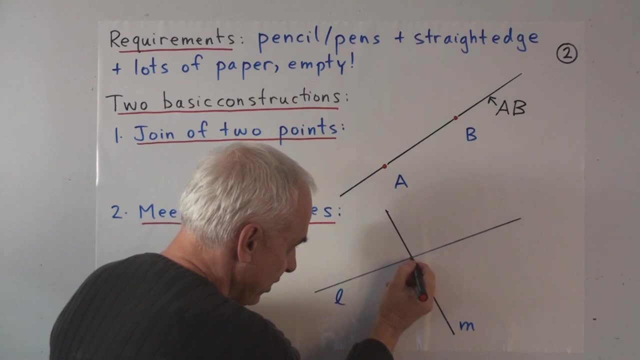 And now the other important construction is what we can do with two lines. This one is simpler because we're just going to draw a point: The two lines meet at a point and we're going to construct that point just by making a point right there. 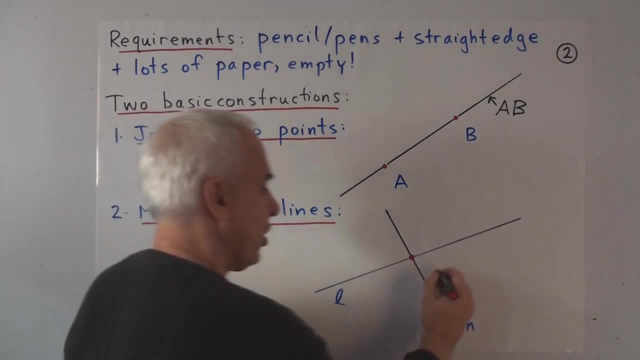 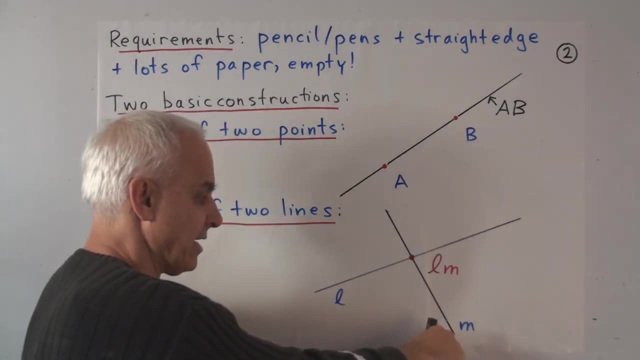 And we'll give that point a name. Let's call it L? M, Because it's created from the two lines little L and little M. So these are the two basic constructions. We use these constructions over and over again And it's not much of an exaggeration to say. 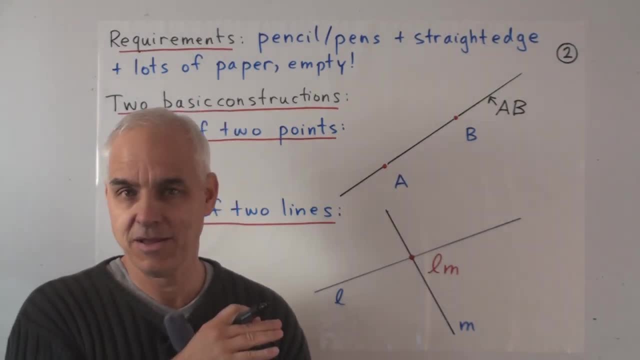 that these are the only constructions that we use in projective geometry, in the plane. We're not going to do any measuring, We're not going to do any perpendicularity constructions, We're not going to use a compass as in Euclidean geometry. 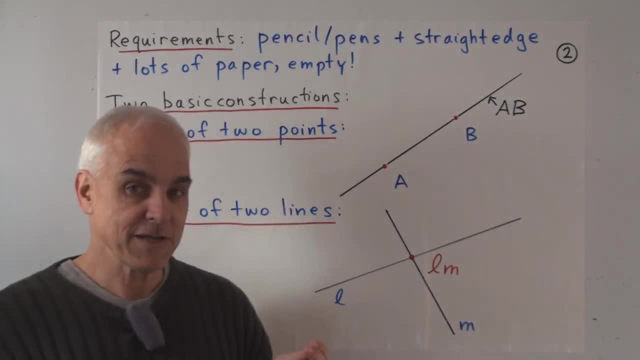 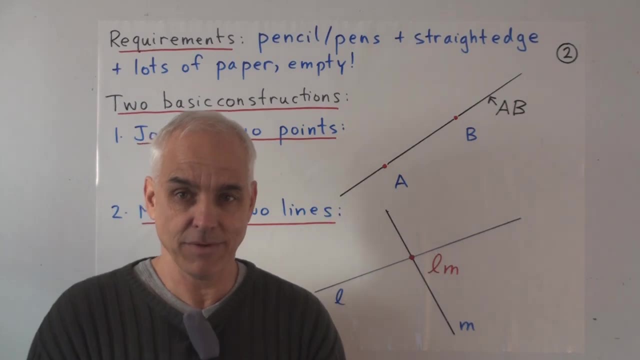 We're just going to stick with points and lines. So it is a very elementary geometry and you might think, well, there's not much that we can do with just such elementary tools, But you'd be very mistaken in thinking that. So here are two very natural and important definitions. 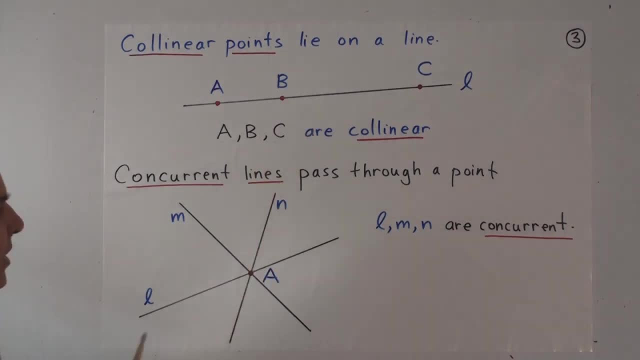 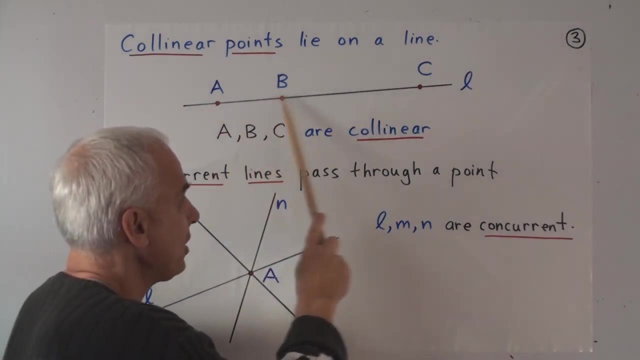 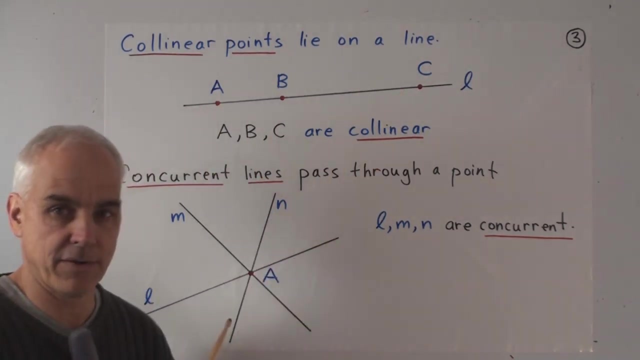 relating to points and lines. The first is the idea of collinear points. If we have a bunch of points which all lie on a single line, then we say that those points are collinear. They share a line. So here A, B and C are collinear. 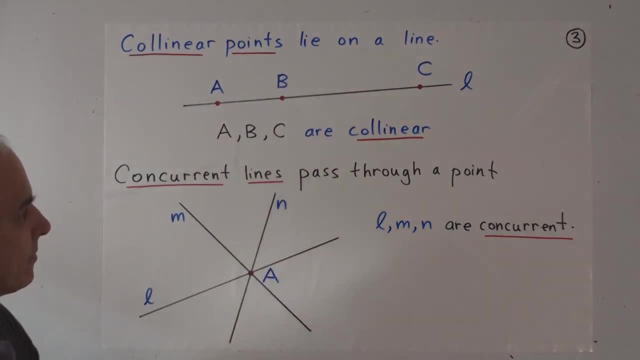 because they're all lying on this line L And we can have more than three points which are collinear. For example, we can make a fourth point there, D say, and then we would have A, B, D and C all collinear. 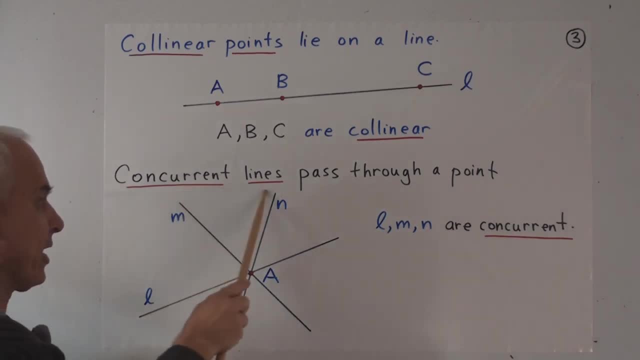 Dual to that is the notion of concurrent lines. This is the idea that concurrent lines are those that pass through a common point. Here we have three lines- The line L, the line M, the line N- And they're concurrent because they all pass through this point A. 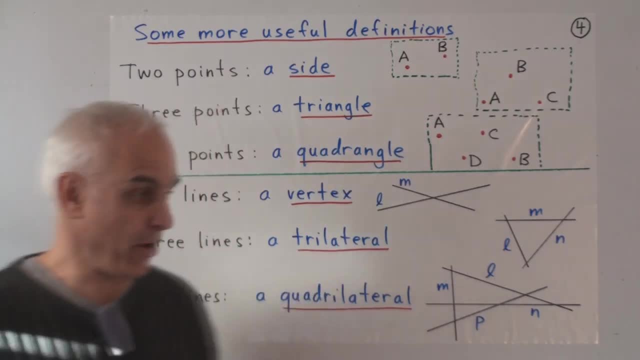 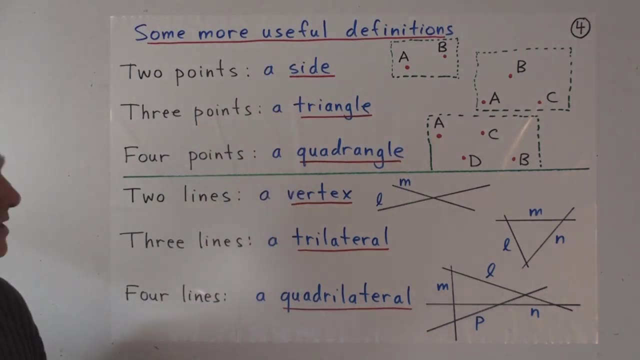 We need a few more definitions before we can get properly going. If we have two points, that configuration of two points we will call a side. So here are two points and that forms a side. Three points form what we call a triangle. So here are three points: A, B and C. 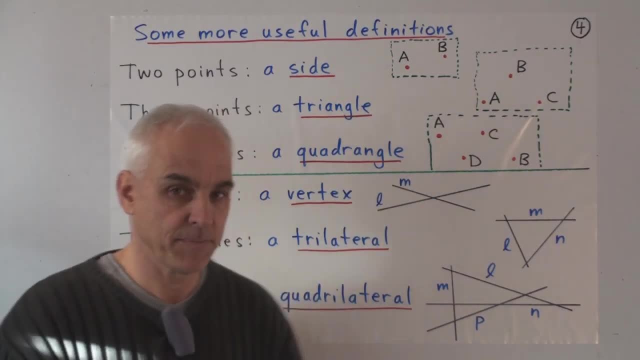 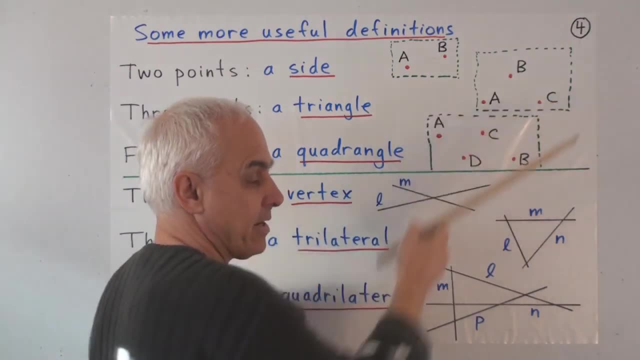 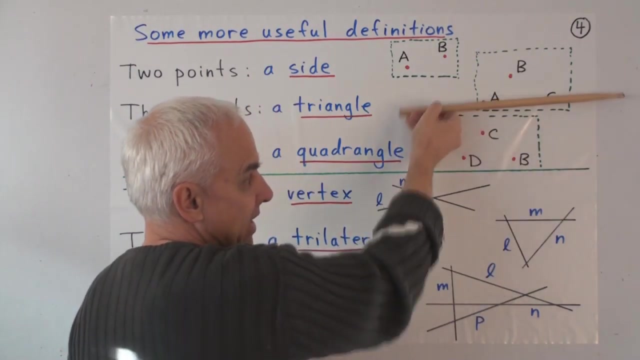 That collection of three points is a triangle. Now, sometimes you might think, well, a triangle should include the sides. And given those three points, yes, we can draw the lines joining A and B, B and C and A and C. 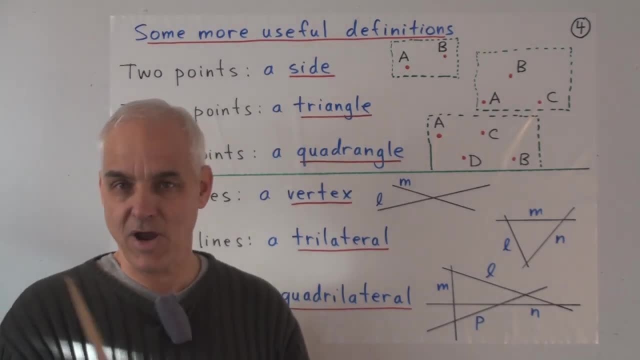 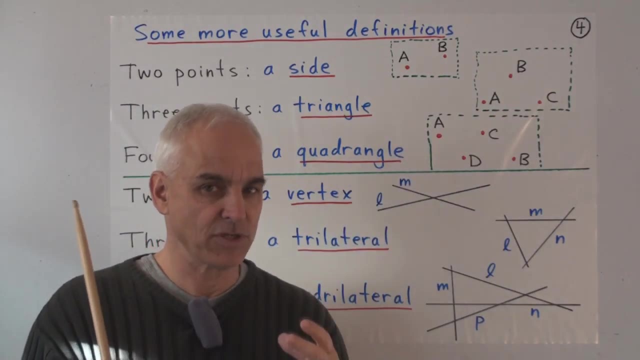 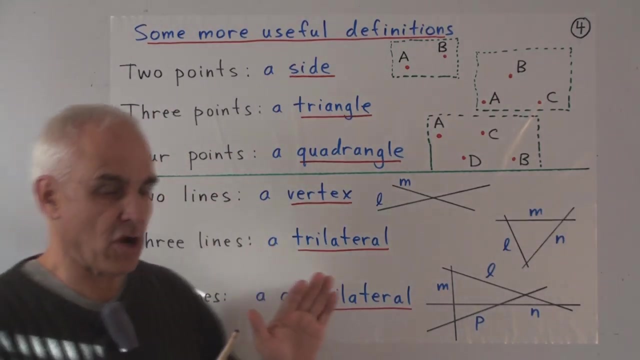 And then we would get something that looks more familiarly like a triangle. But it's convenient for us to think of the official definition of a triangle As just being those three points. Sometimes the special case when the three points are collinear is excluded from the definition of a triangle. 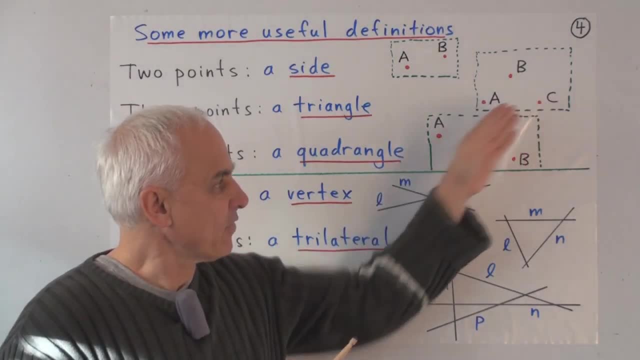 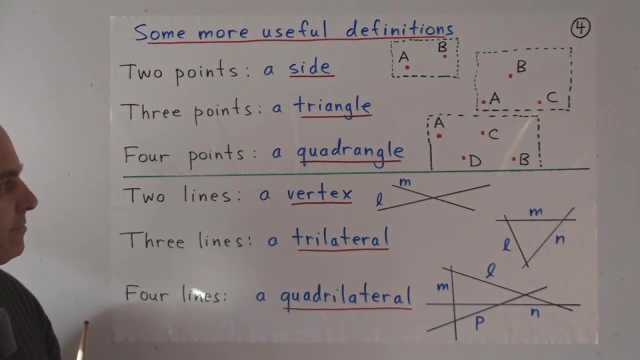 And we'll generally say that if the three points are collinear then we have a degenerate triangle. It's not a real triangle. Going up one step to four points. four points gives us what we call a quadrangle. So four points: A, B, C, D. 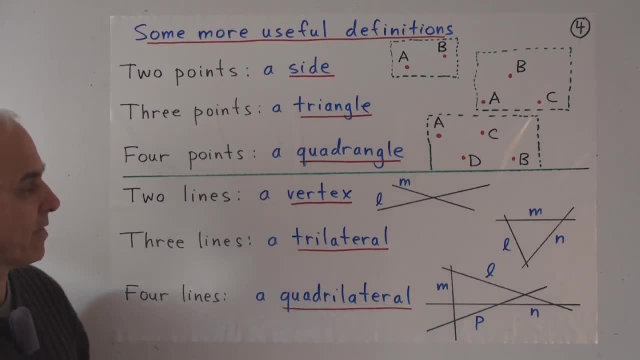 in the plane form: a quadrangle, Side triangle, quadrangle, Natural hierarchy of arrangements of points Dual to that, we have three notions relating to lines. If we have just two lines by themselves, we say that configuration is a vertex. So this configuration of two lines is a vertex. 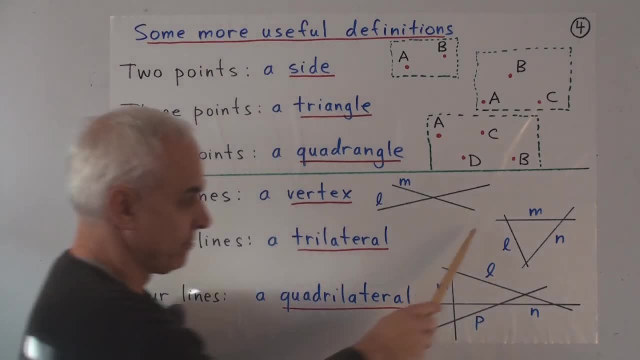 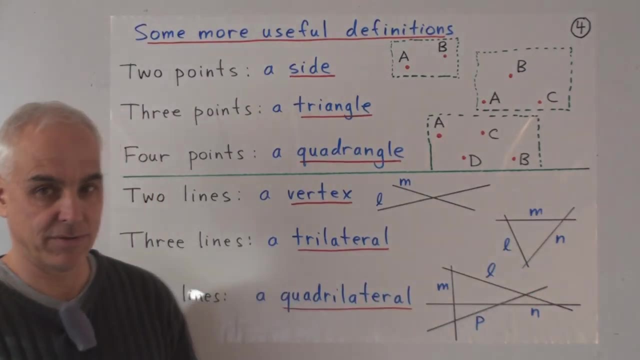 If we have three lines, like L, M and N, then we say that configuration is a trilateral- Almost the same word as triangle, but different. So a triangle is three points, a trilateral is three lines And in projective geometry 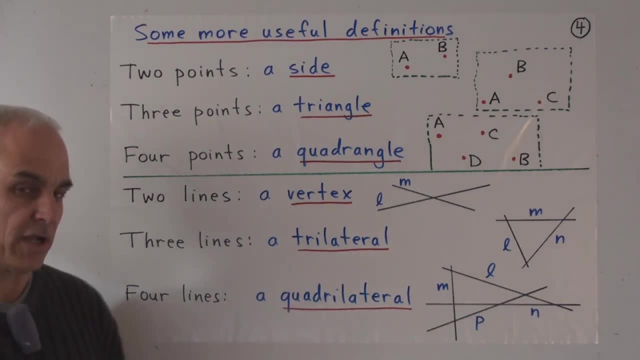 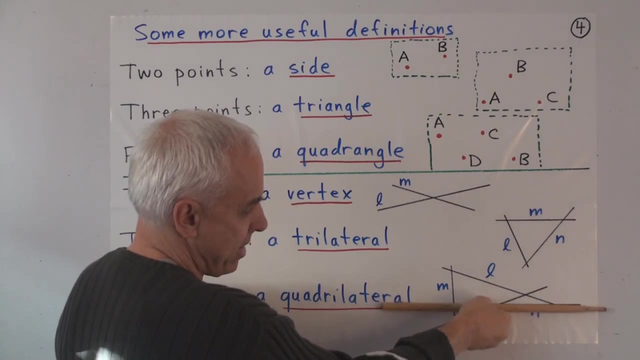 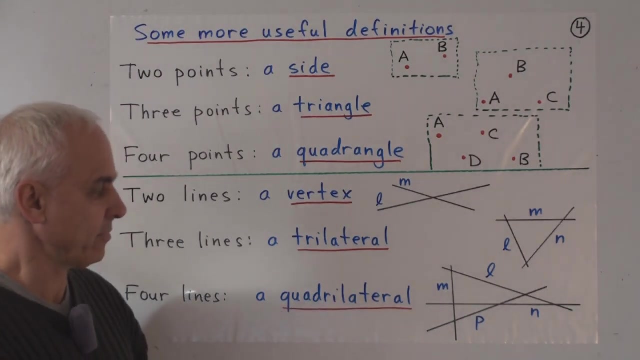 if you have four lines, that configuration is called a quadrilateral. So here we have four lines: L, M, N and P, And they can be more or less wherever they want to be. That's a quadrilateral Now, just as over here with the triangle. 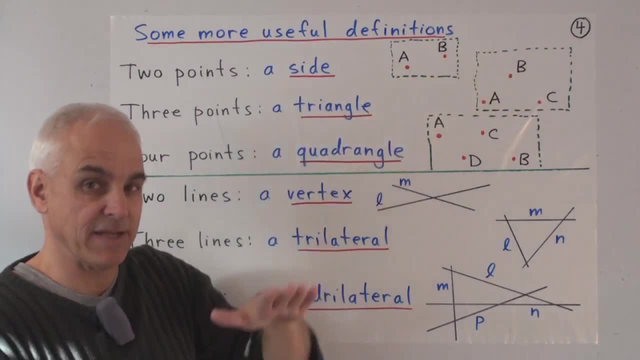 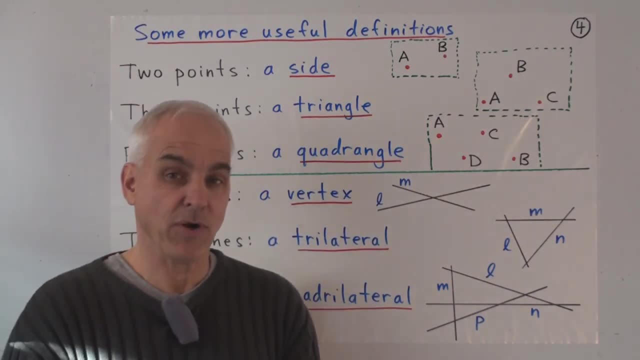 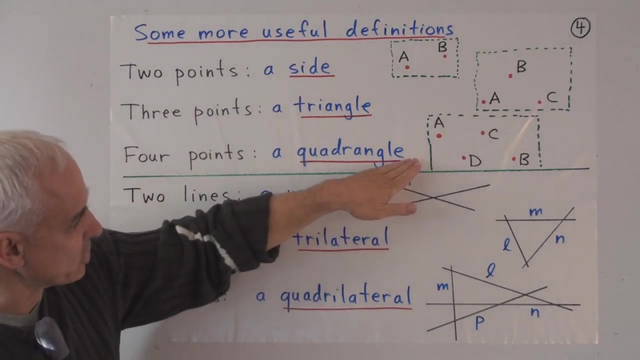 we said that if the three points are collinear that's a degenerate case. so also with the trilateral. If the three lines are concurrent, then that's a degenerate trilateral, And there's also notions of degenerate quadrangle. 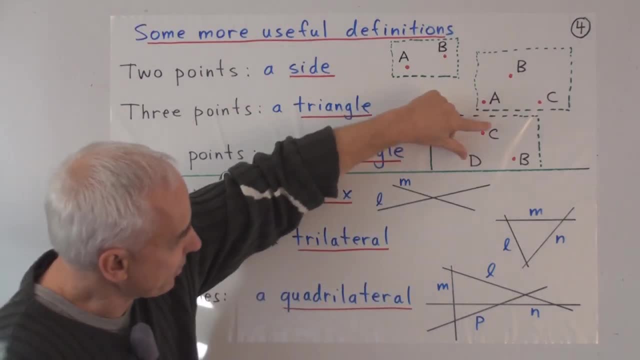 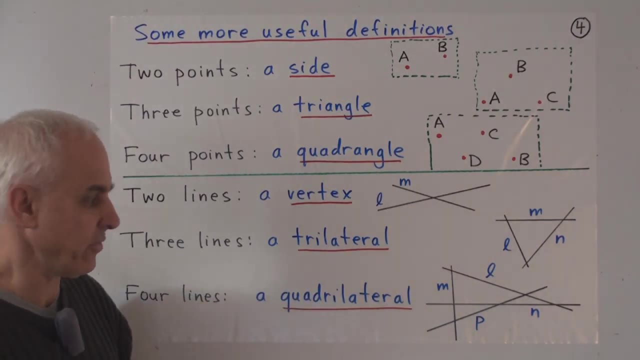 and degenerate quadrilateral. So when three of the four points are collinear- that's sort of a special case- We sometimes say the quadrangle is degenerate. Or if three of the four lines in a quadrilateral are concurrent, we can also say that the quadrilateral is degenerate. 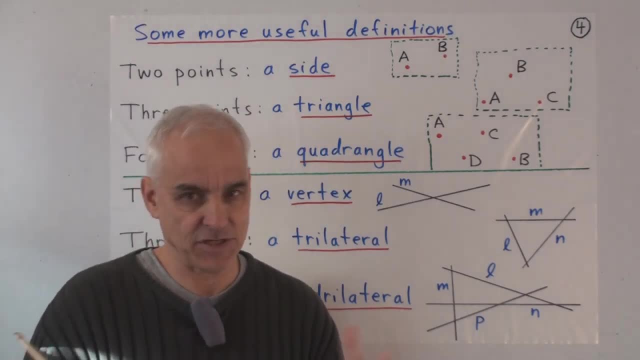 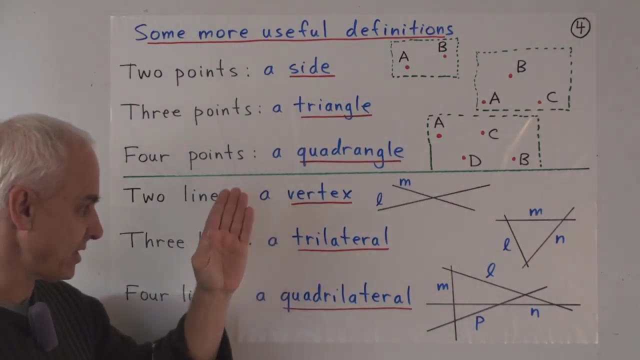 But we're not going to really worry about such things. This is just an introduction. So we have sides, triangles and quadrangles of points. We have vertices, trilaterals and quadrilaterals of lines. So it's a terminology. 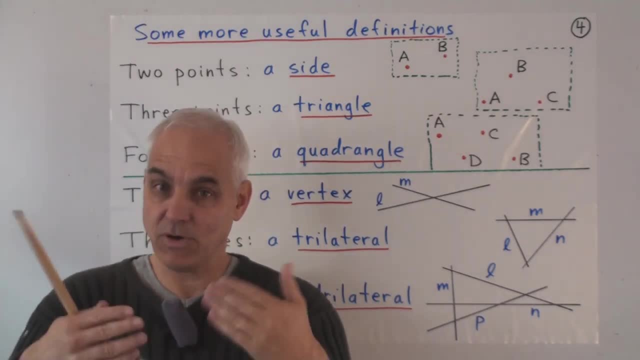 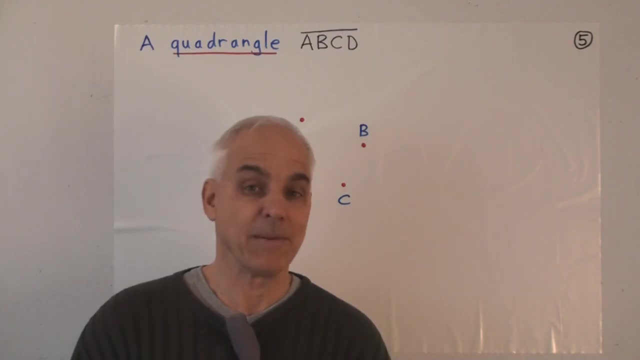 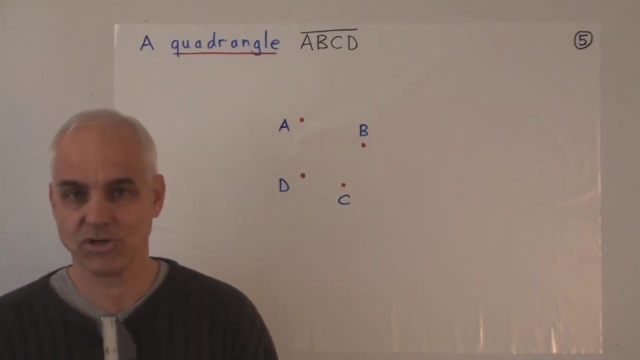 so that we can be consistent and we can understand what we're talking about, you and I. So now let's have a look. what can we do with points and lines? Okay, so let's start doing some projective geometry And we'll start with some points on the page. 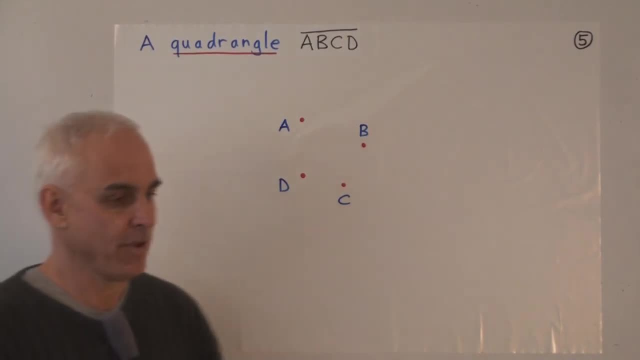 So get yourself a big sheet of paper- Eight and a half by eleven is fine- And draw a few points, say four points in the generally in the middle of the paper, And it's probably not a bad idea if you organize the four points. 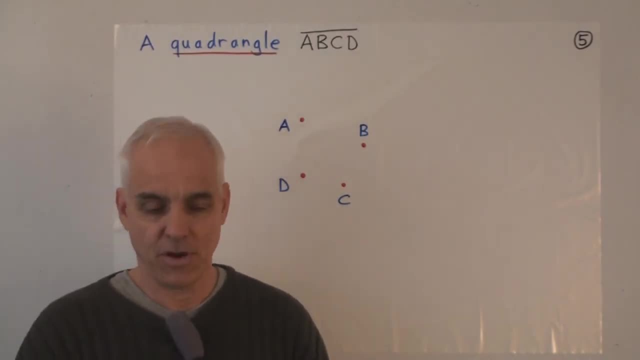 so they look something like these ones, Okay, and I ask you to follow along and do the same constructions that I'm doing, And we're interested in accuracy. We're interested in making sure that our lines are straight and that they really do go right through any two points. 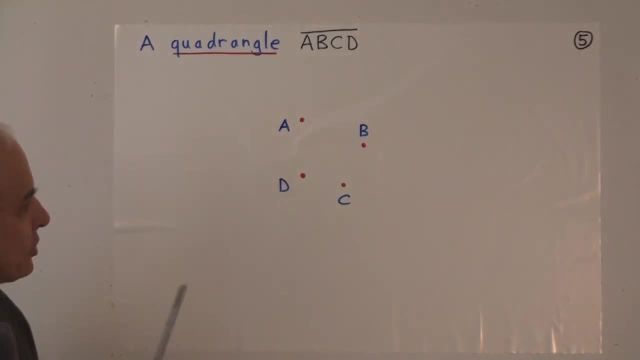 that we're drawing. So if we start off with just one point A, then there's not much to do. If we have two points- A and B- there's really only one thing we can do. So let's do it If we just have A and B. 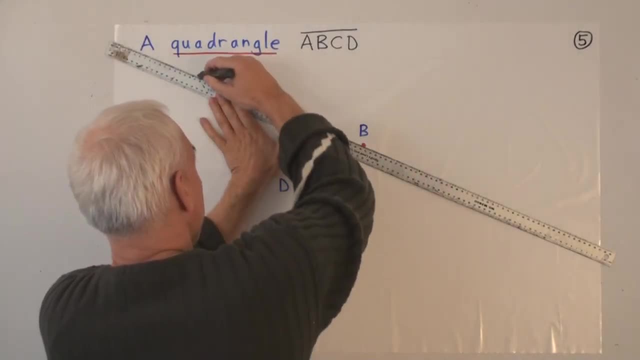 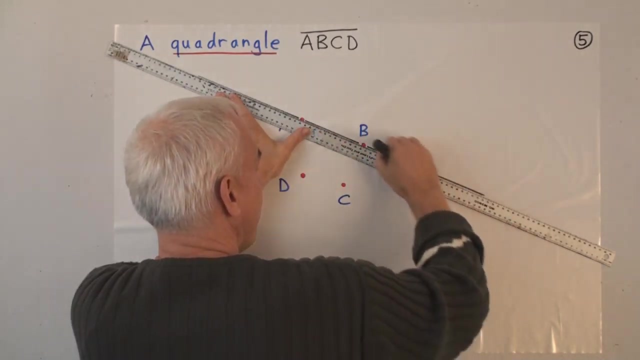 what we can do is we can draw the line through A and B. So I'm going to line them up, I'm going to avoid the points so we can see them still, And our lines, how long they are. well, they're kind of variable. 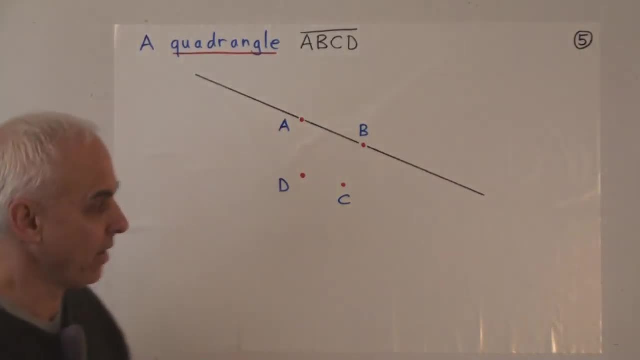 We can always extend lines if we need to. So the lines that we are drawing are always finite, of course, because the paper is just finite, But we imagine that the lines can be extended if they need to be, So, with two points. 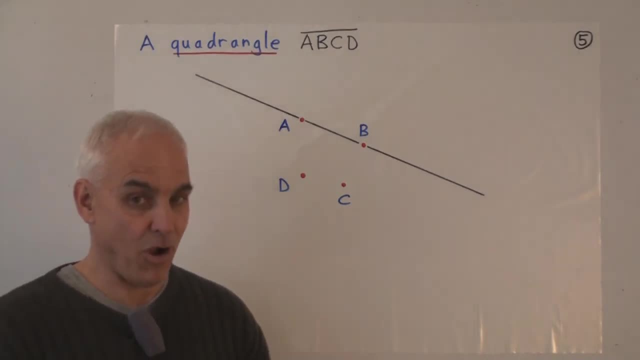 we can join the two points to form a line, and that's about all that we can do. Now let's add a third point. Well, if we have a third point, then we have some more lines that we can draw. We can join B and C. 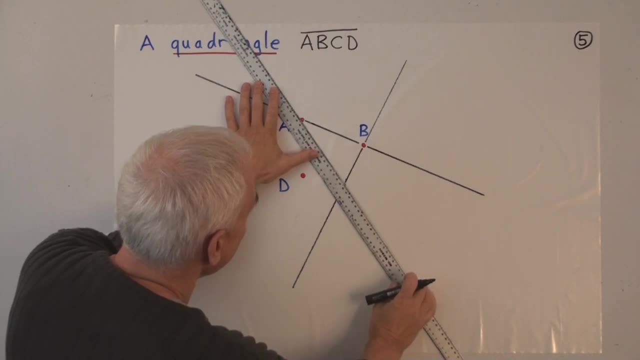 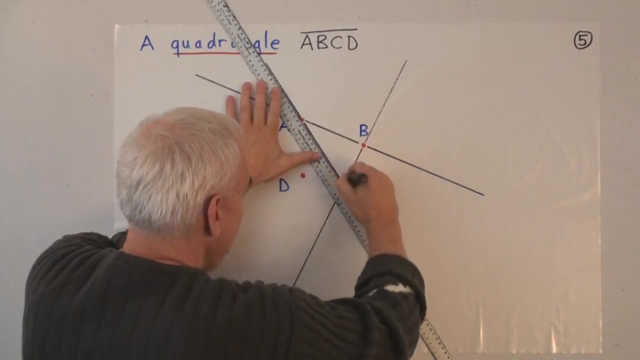 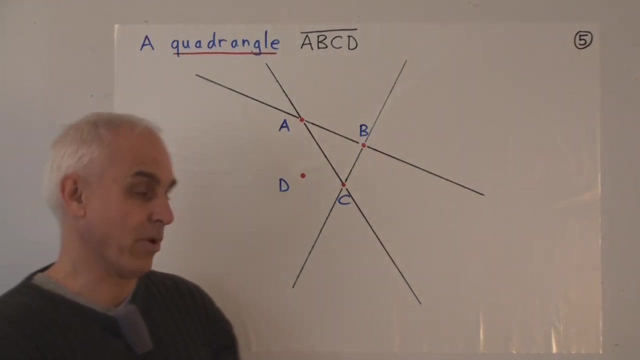 And we can also join A and C. So please do that on your paper, making sure that you go right through the middle of the points and that you're not moving your ruler. So with three points or a triangle, we can form an associated trilateral. 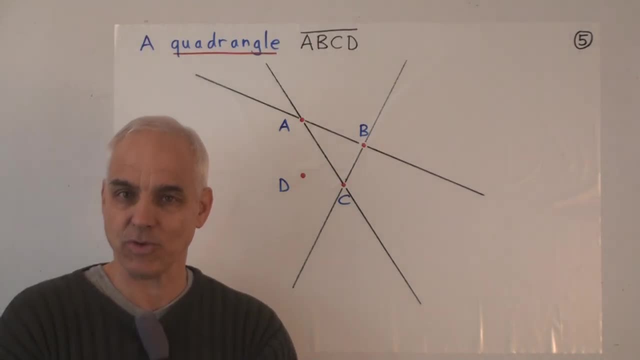 We can draw the three lines determined by those three points, And after we've done that, then that's pretty well it. There's not much more. we can do with those three points and three lines, But with a fourth point all kinds of beautiful possibilities emerge. 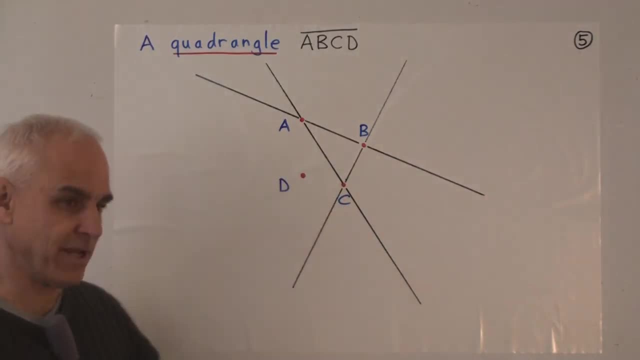 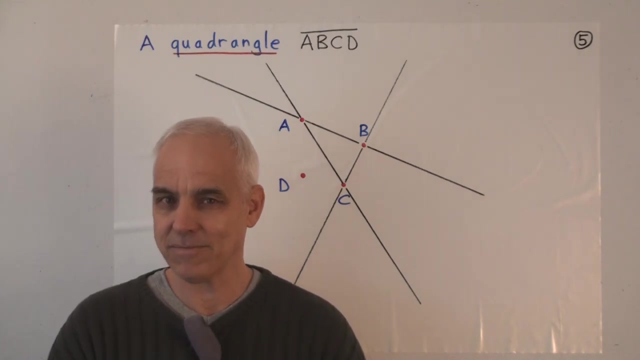 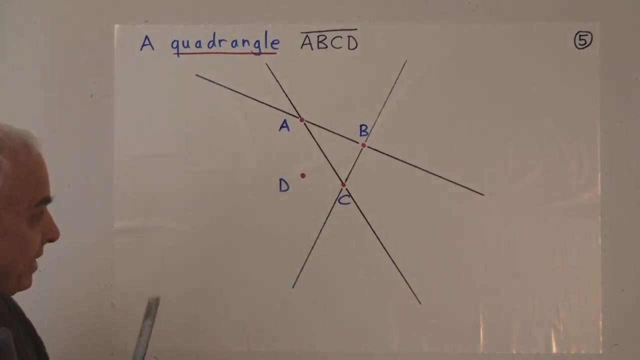 So from three points, which is rather limited to four points, is a whole lifetime of study. Let me see if I can convince you of that possibility. So we're adding one more point D to the three points A, B and C. 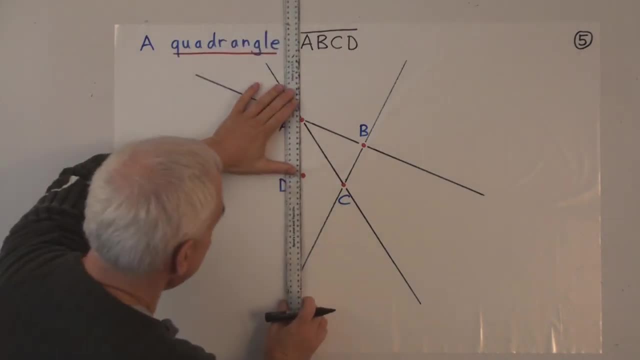 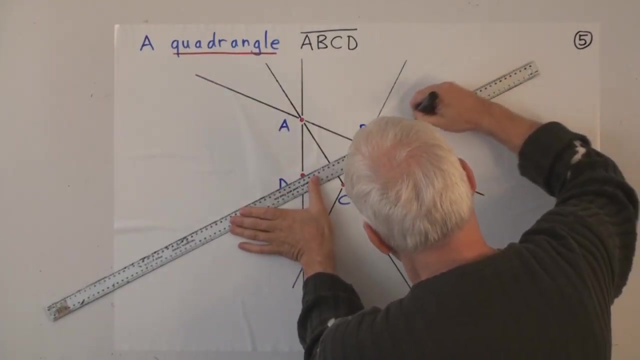 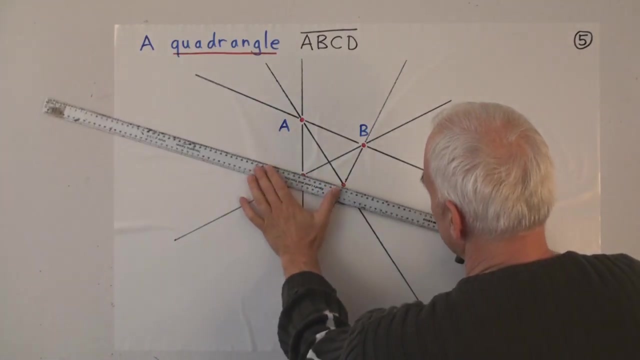 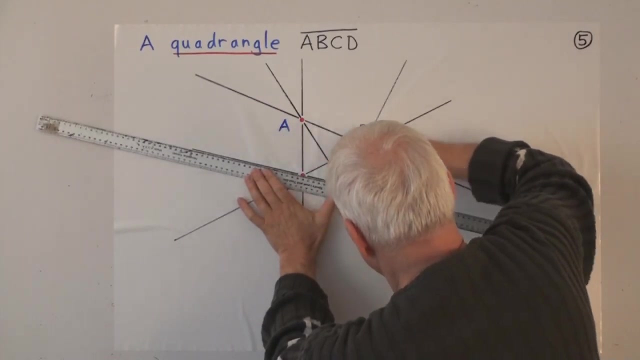 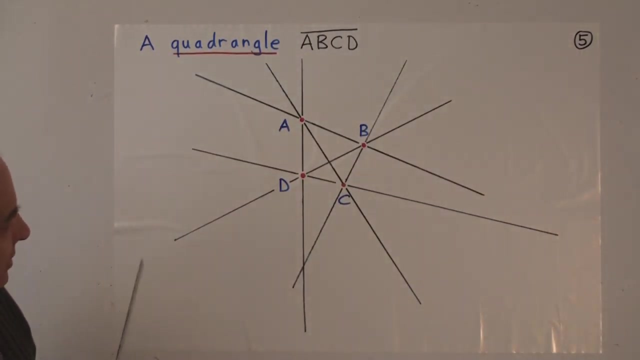 So now we have some more lines to draw. We can connect A and D, We can connect B and D And D and C, And now we see that we've got six lines. So the four points determine six lines. Can you see those six lines? 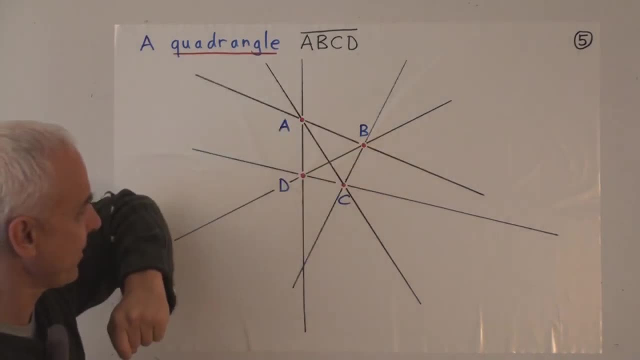 Let's make sure we see them. So there's A B, There's A C, There's A D, There's B C, There's B D And there's C D, So we started off with four points. 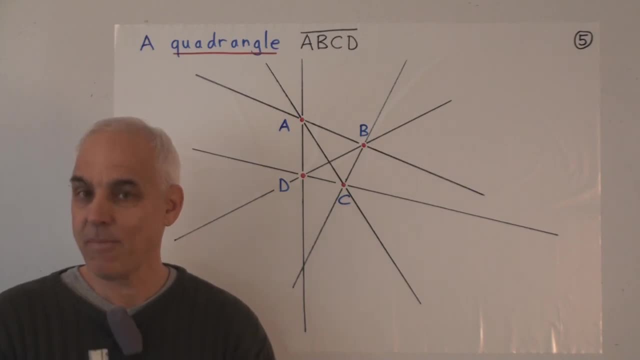 and now we have six lines, But we have something else, Because those six lines meet in a couple of new points. We're getting a new point right here And we're getting a new point right here. Any other new points? Well, there is another new point. 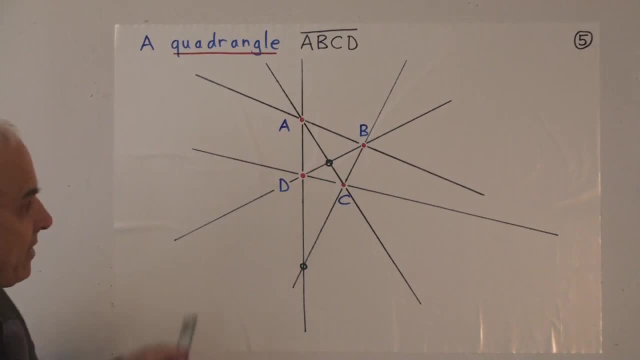 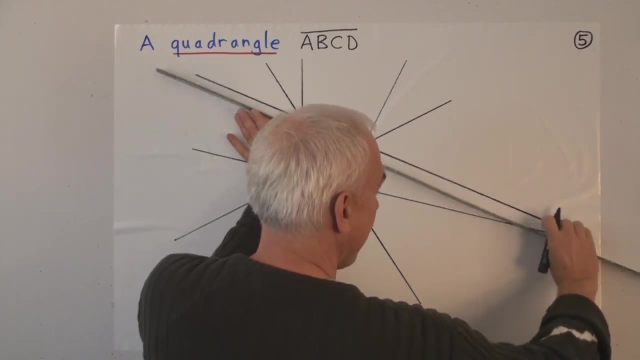 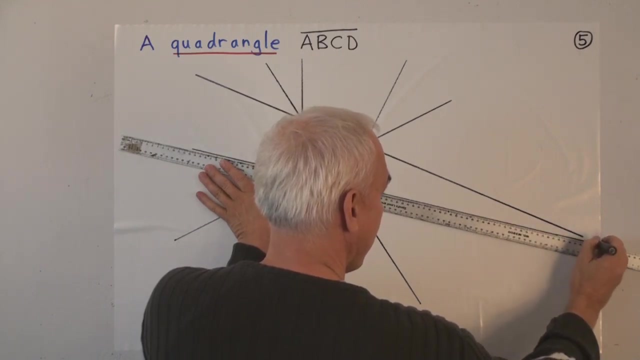 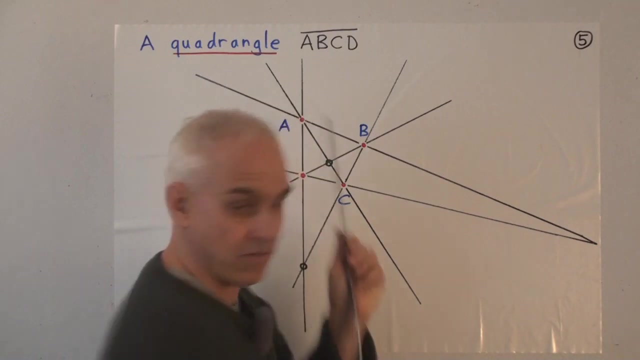 But I need to extend my lines a little bit to see that point. So I need to extend this line a little bit And this line a little bit And it looks like we're getting our third point just at the end of the page there. 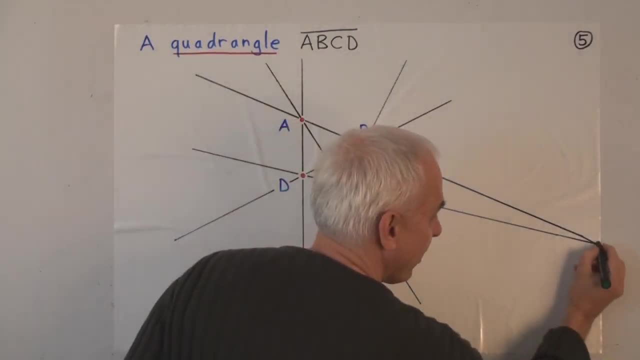 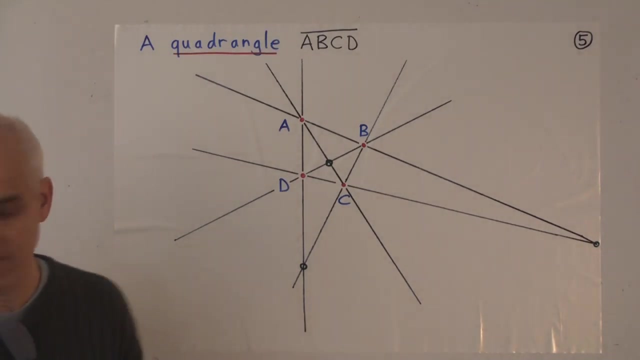 So there's another new point. So we started with, say, we started with four points, And then we get six lines, And now we see that we also get three new. well, let's call them diagonal points And maybe I can give them some names. 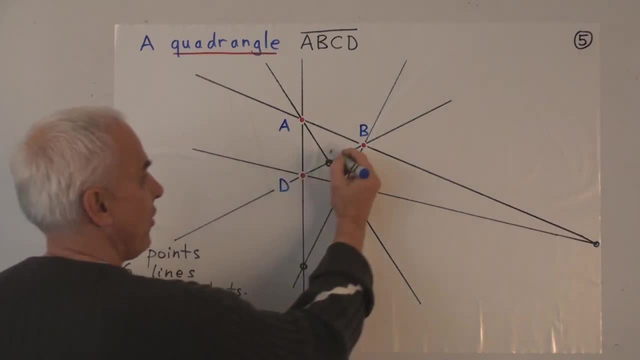 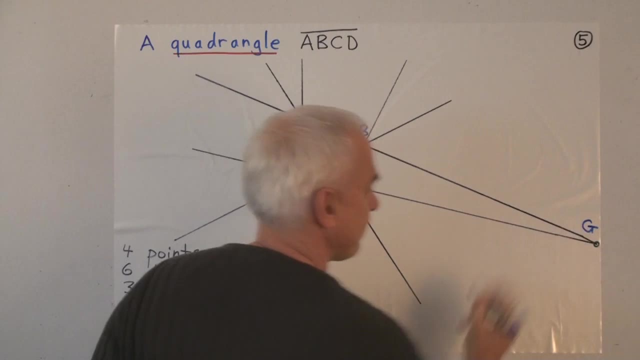 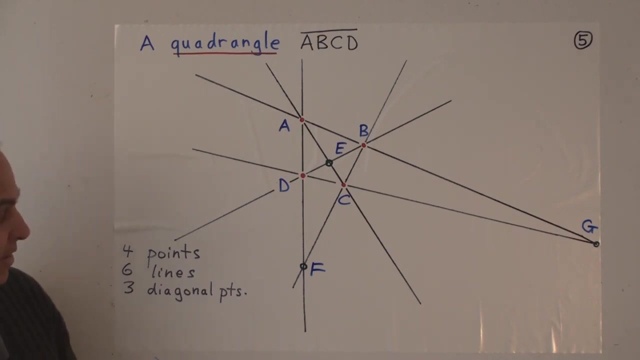 What should we call them? Let's call this one E And F And G over here. So we started with A, B, C, D, We've drawn our six lines connecting them And we get three new points: E, F and G. 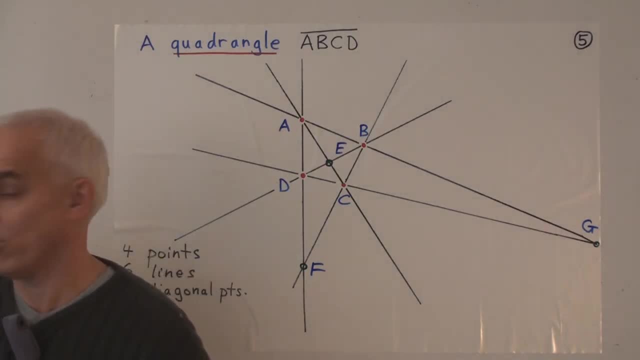 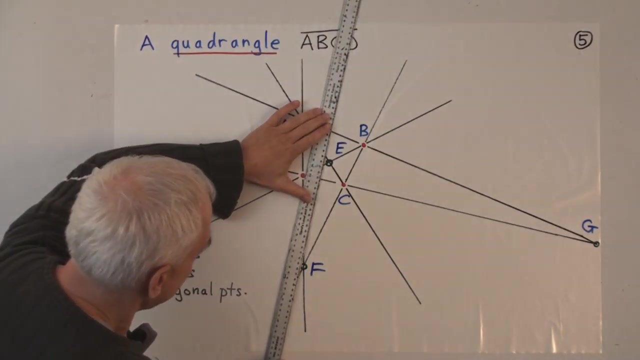 Which we can call diagonal points. So what do you think we can do now? Well, whenever we have two points which are not connected with a line, we can connect them with a line. So E and F can be connected with a line. 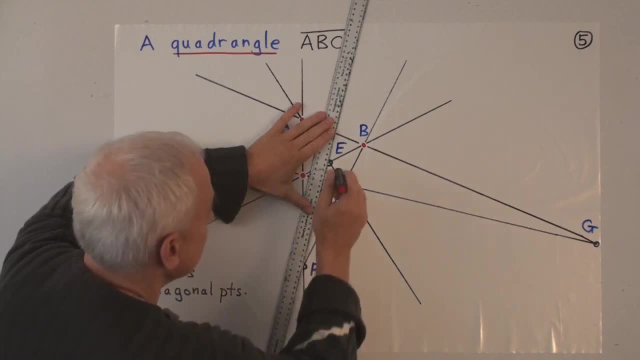 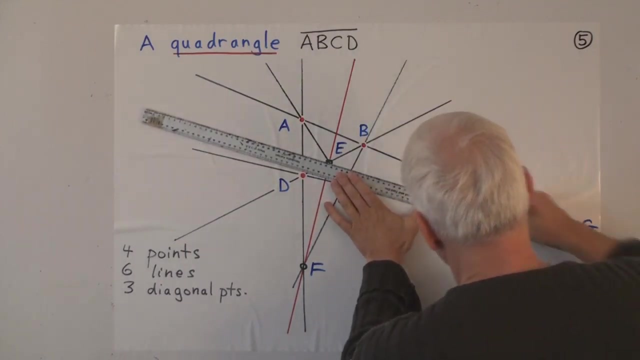 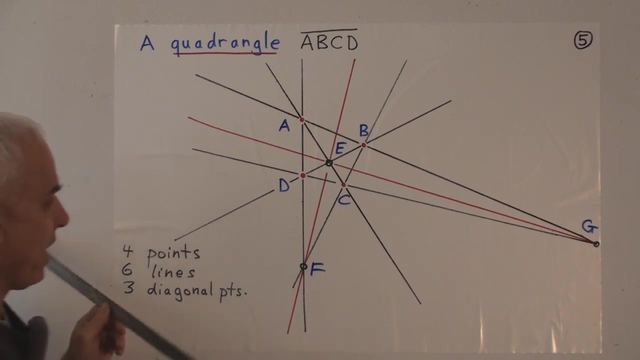 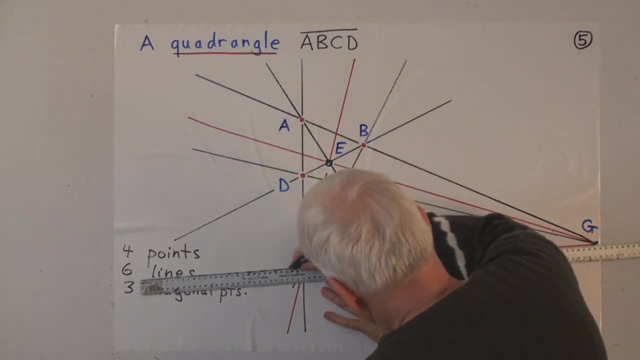 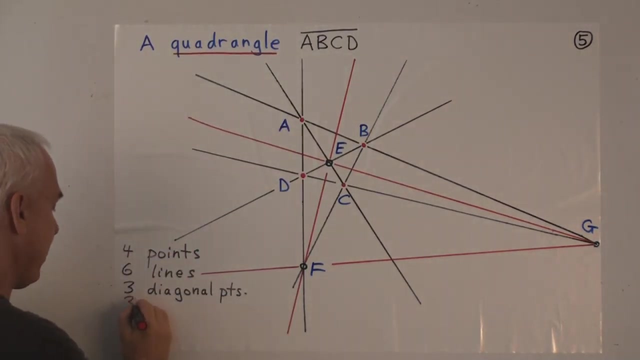 And let's do that. I'll do it in red here. So there's a red line going through E and F, And then we want a line through E and G And also through F and G. So we now have three diagonal lines. 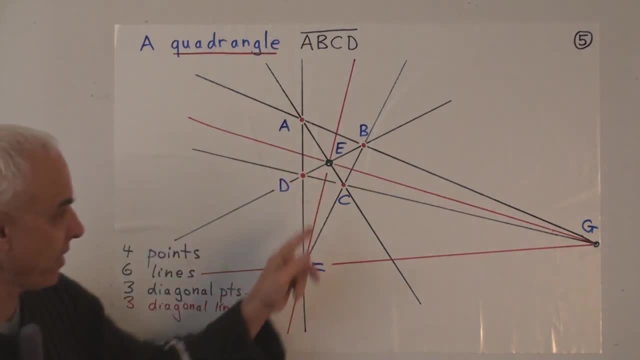 We can call these red ones diagonal lines. So we started off with four points, Then we got six lines, Then we got three diagonal points- E, F and G- And now we've created from those three diagonal points three new lines. 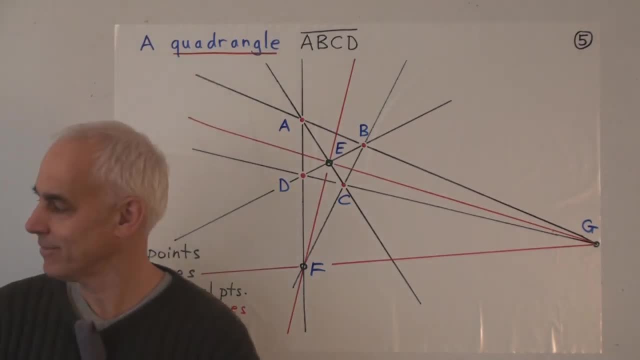 which we'll call diagonal lines. So what can we do now? Are there any more points that we can join? I don't know, All the points that we have created are now joined, But the other construction that we can do is we can find the meet of lines. 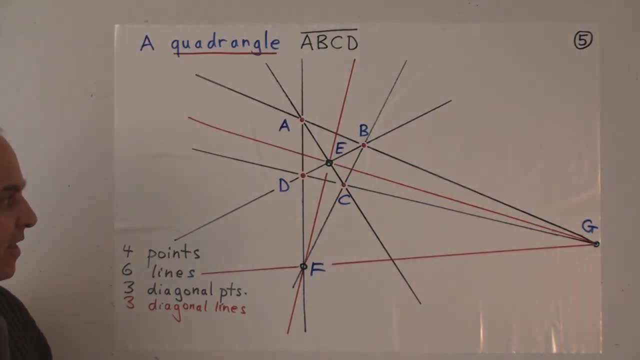 Are there any new meets of lines that are appearing? Well, yes, there are. These new red lines that we've just drawn meet the black lines in some new points, And let's see if we can find them all. So this red line here meets this black line. 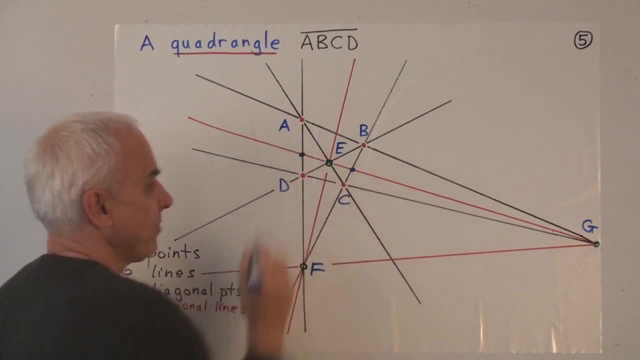 and this black line in these two points, And this red line meets this black line and that black line in two points there. And then we have this red line which meets this point. there. There should be a second point, shouldn't there? Where's that second point that it meets? 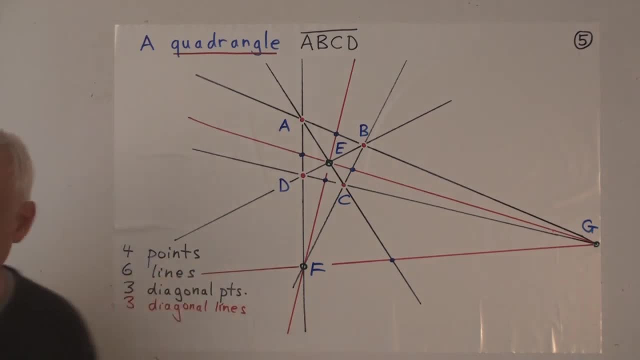 Ah, it's going to meet this black line over here somewhere over there. We need to extend the lines a little bit to see that Maybe it's going to go off the page. Let's see. So we'll extend this sort of through there. 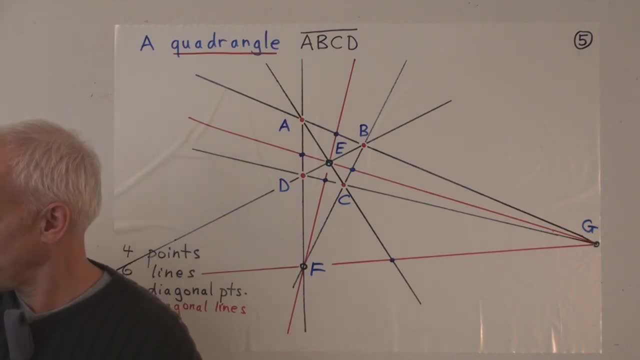 And we'll extend the red one. Okay, so there's another point somewhere right about there, Another blue point which is a little bit over in that direction. So we have six new points: One, two, three, four, five, six. 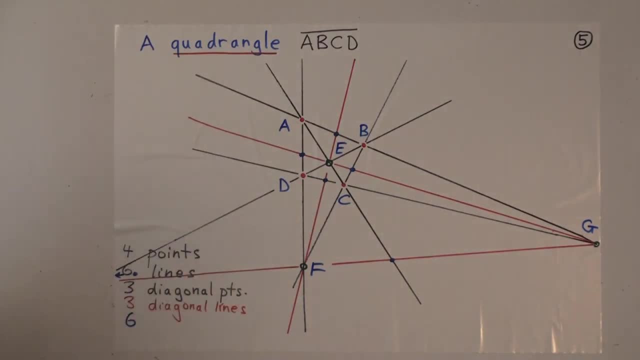 Six. Let's just call them new lines. They're not lines, they're points. Six new points, All right, good, What can we do now? Well, those six new points can be joined, And we might use green, Okay. 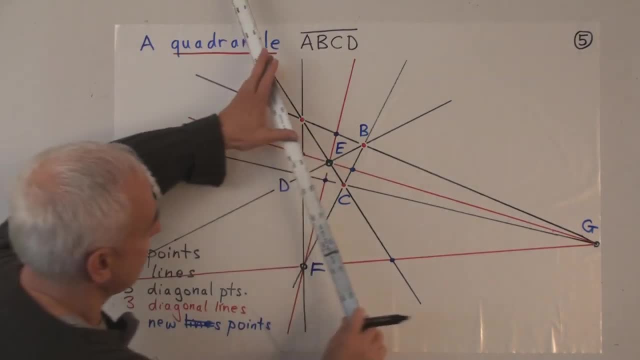 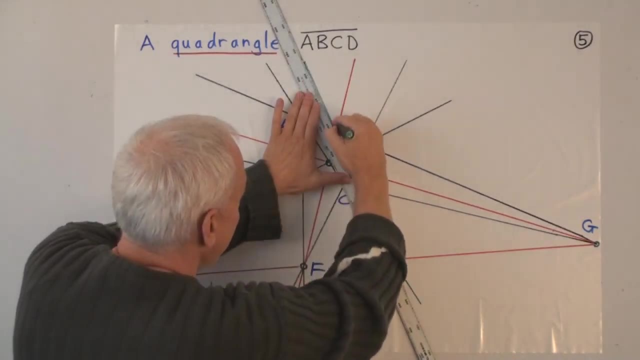 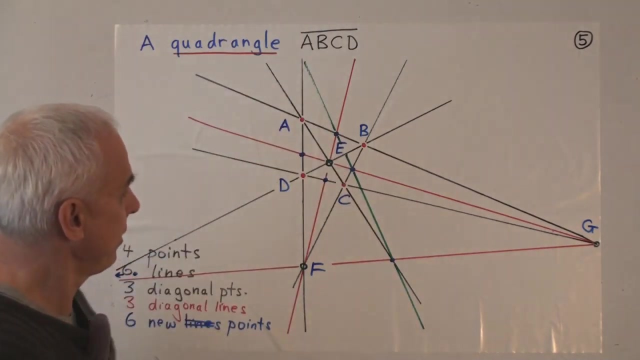 So let's have a look at, say, these two blue points, We can join them, Keep going, Now we go. hey, wait a minute. How come the line joining those two blue points also went through that blue point? That seems like a coincidence. 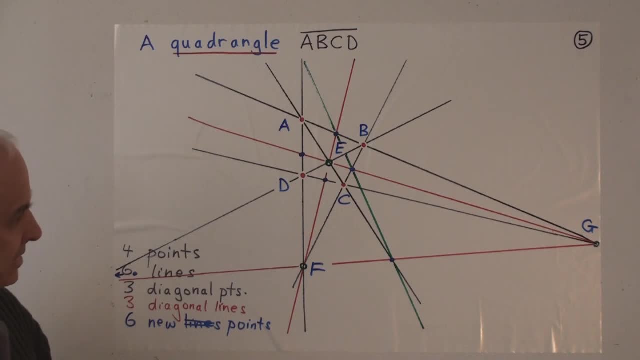 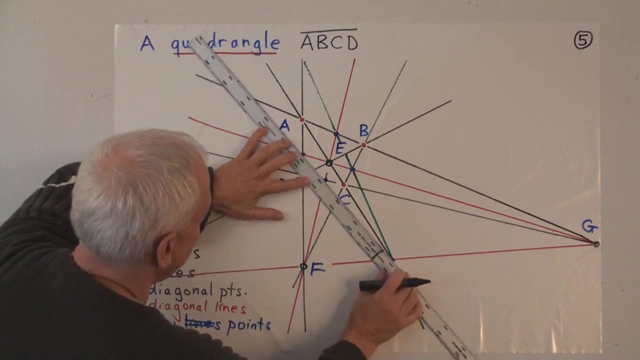 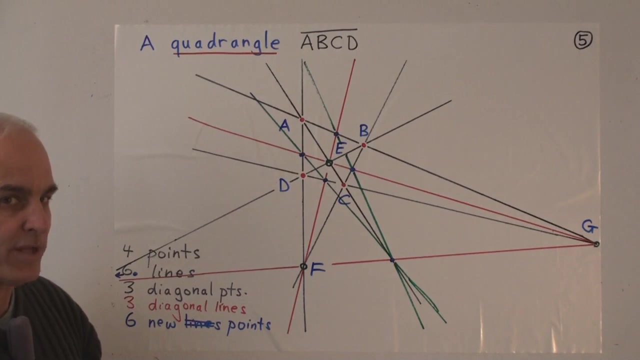 or a bit of a surprise, Let's see what happens- say, with these two points, We can join them. They're not joined yet. Oh, that wasn't too straight. There we go. So we've just joined these two blue points. 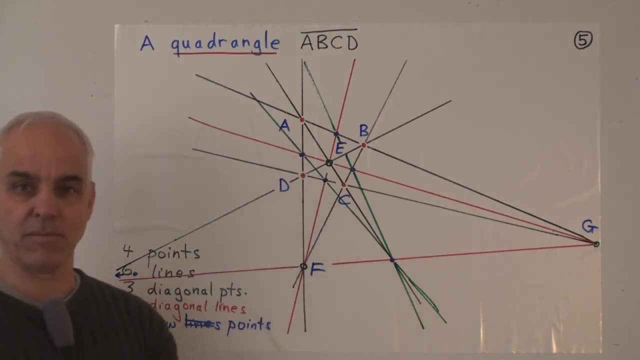 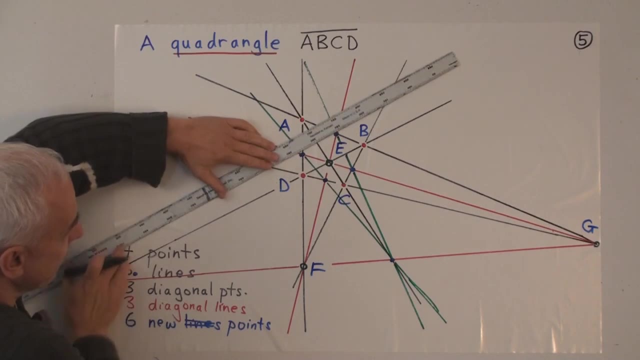 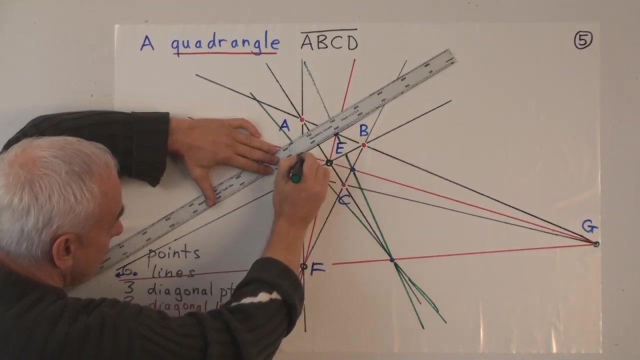 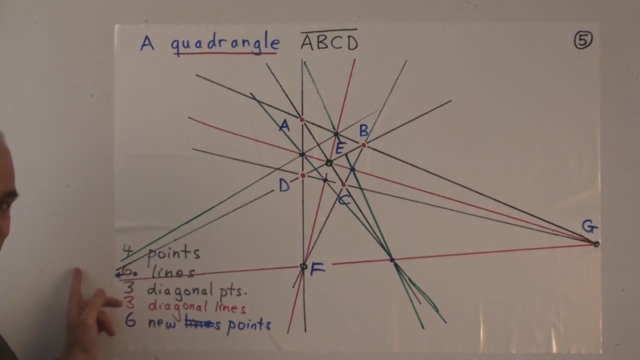 We've gotten another line which also goes through that blue point. That's cool. What about say, joining these two points? That looks a lot like it's going to go through that extra blue point which is to the left here and off the page. 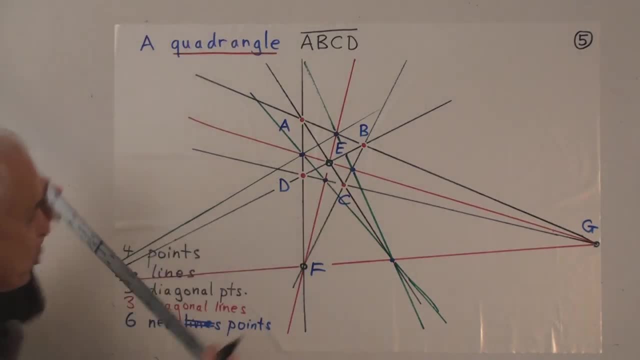 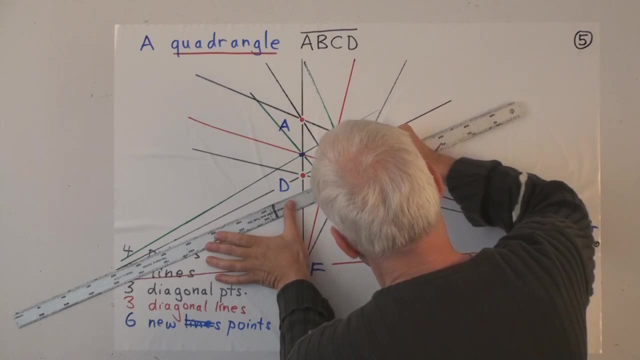 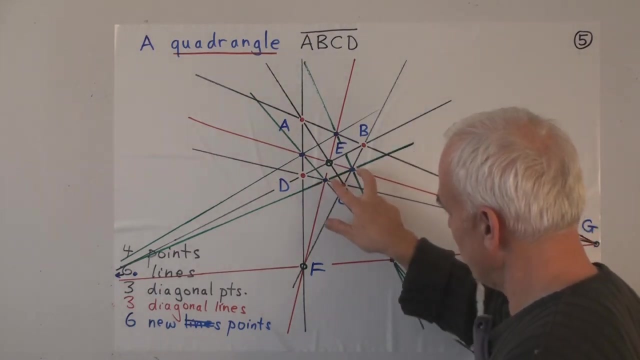 And similarly between these two blue ones which we haven't joined. yet. So this new line that we've drawn between these two blue points also goes through that third blue point on that side. there, And now we've connected all the six new blue points. 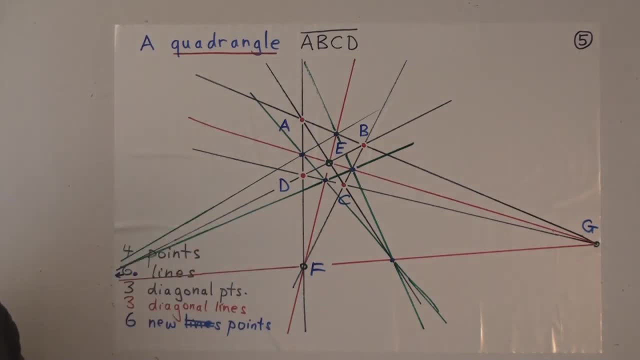 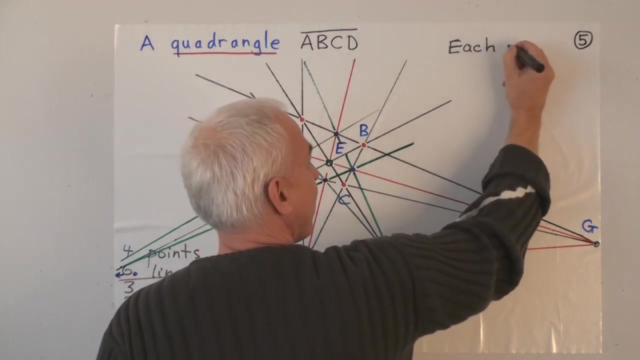 And we've used four new green lines, So we have four new lines. There's something remarkable that's happening here, isn't there? It's rather remarkable that these four green lines pass each through three of the blue points, So each green line. 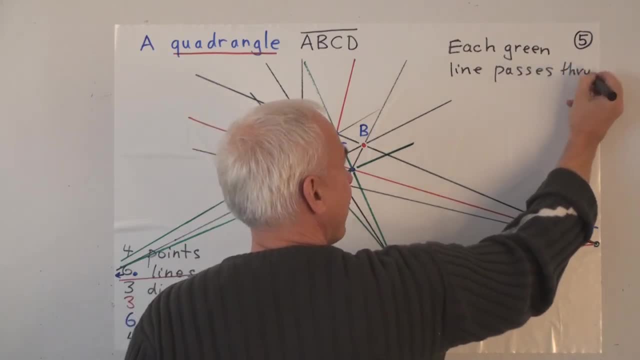 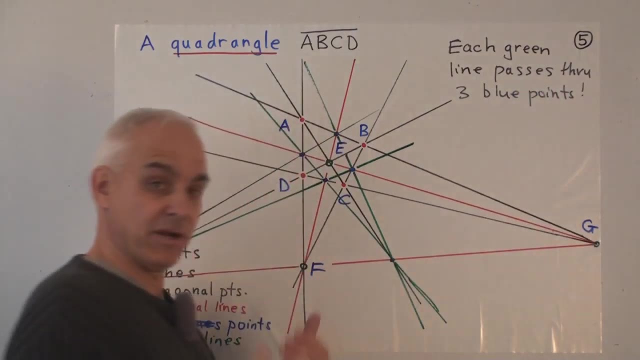 passes through three blue points, Or at least it appears to in this particular case that I have drawn. What about the case that you drew? Did you find also the same thing happening? Well, my guess is that if you did things accurately, you would have found that to be the case. 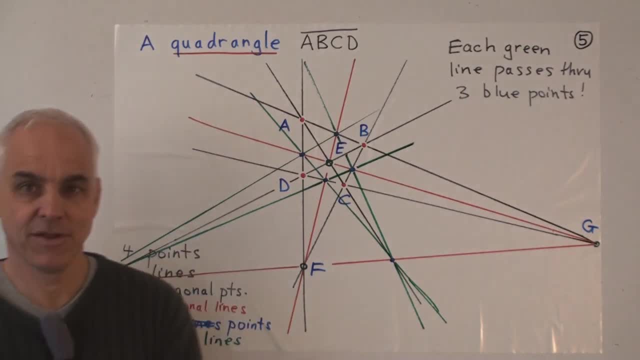 So here's now a new line. So here's now a very interesting exercise To repeat this with a number of different configurations of four starting points And see if the same rather remarkable phenomena takes place. We started out with four red points. Ultimately, we ended up with four green lines. 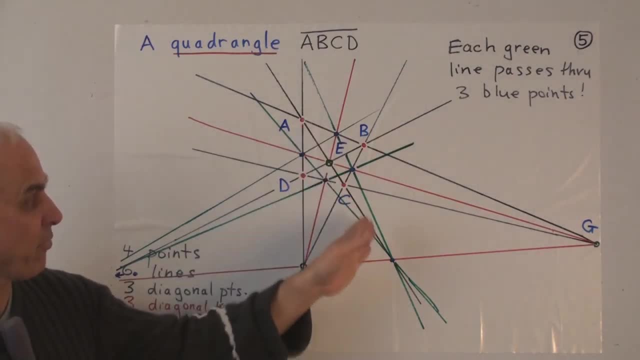 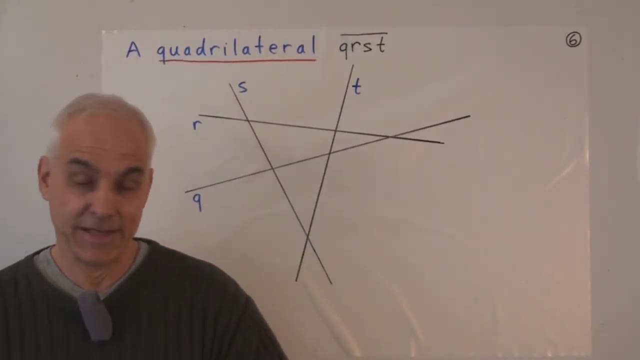 that had a pleasant collinearity property with respect to these six blue points. So that was fun. Let's see what happens if we start with a quadrilateral instead of a quadrangle, If we start with four lines rather than four points. So here's a quadrilateral. 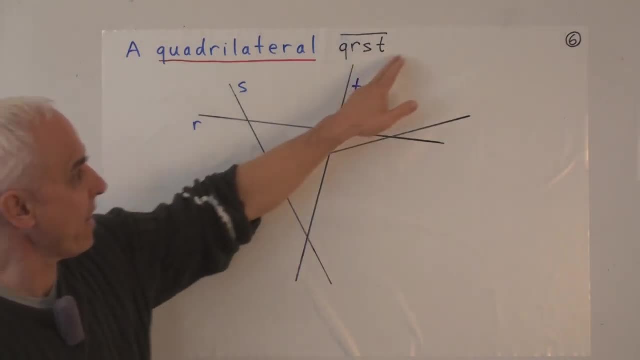 It's called lines QRST. This is sort of my name or expression that we're going to use for a quadrilateral. There's a line Q, There's a line R, There's a line S And there's the line Q. 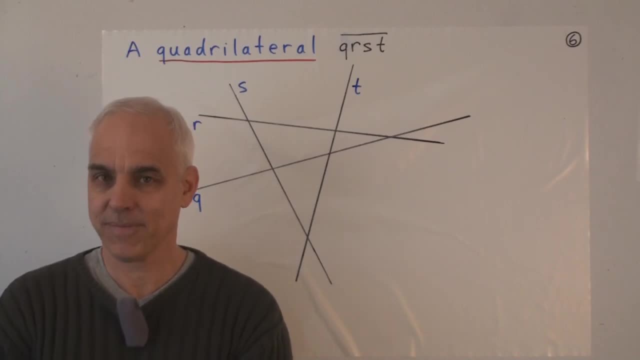 And T, Four lines we're starting with And now we're going to just do projective geometry constructions. Whenever we have a line, let's say Q. there's not much we can do with it. If we have two lines, say Q and R. 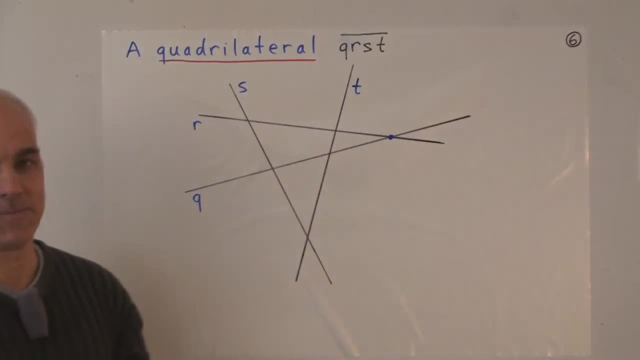 then we can. we can find their meet. If we have three lines, say Q, R and S, then we have two additional meets. We then have a trilateral of lines and a triangle of points, But with those three lines and three points. 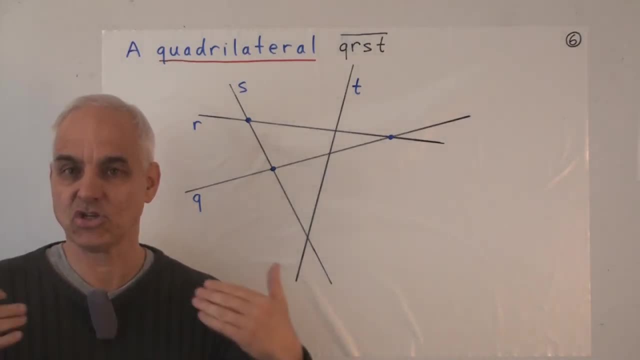 there's nothing else that we can do, Our constructions stop. However, with a fourth line, then we have a whole universe of possibilities opening up in front of us. So we add this fourth line, Giving us three new points. So the four lines that we started with. 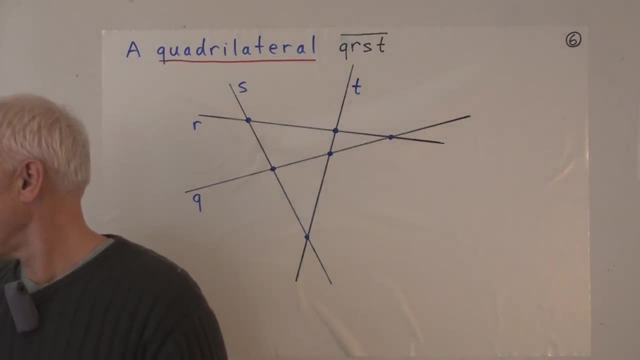 give us six points. So let's record that We started with four points, With four lines actually, And they were in black, so maybe I'll do it in black: Four lines, And then we have six points Determined by those four lines. 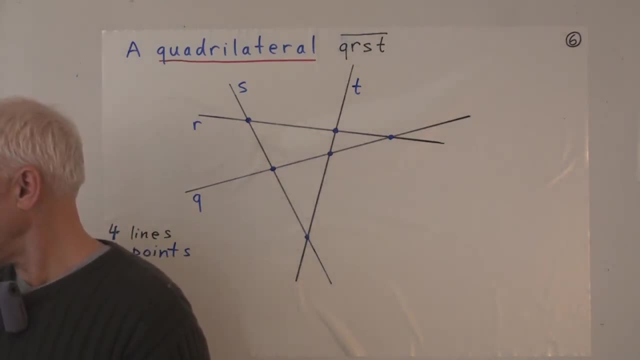 Alright, what can we do now with these six points? Well, we can join some of them. Some of them are already joined, But we can join the ones which are not already joined. For example, this point and this point are not yet joined. 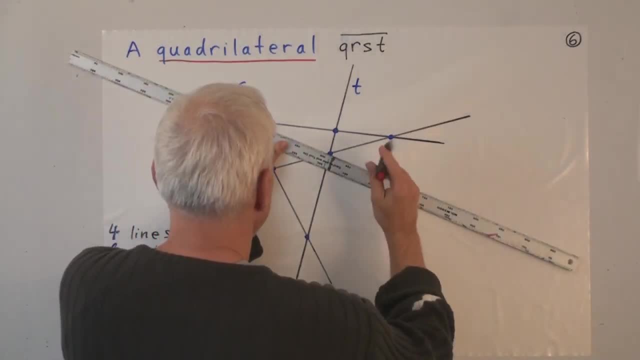 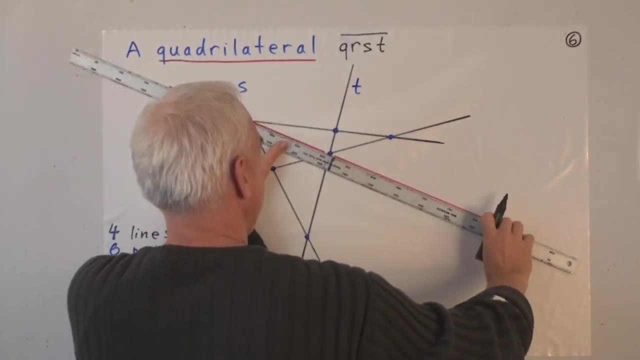 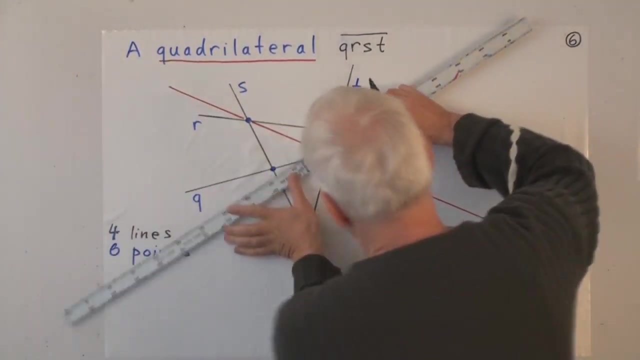 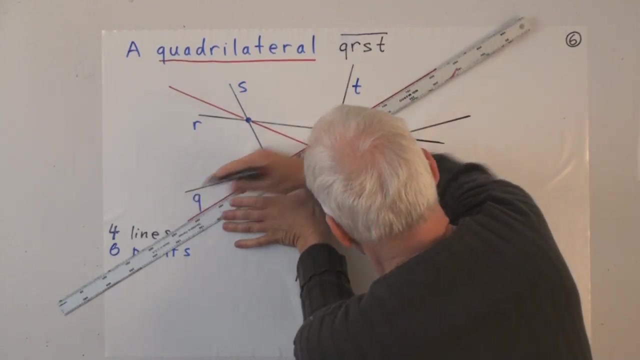 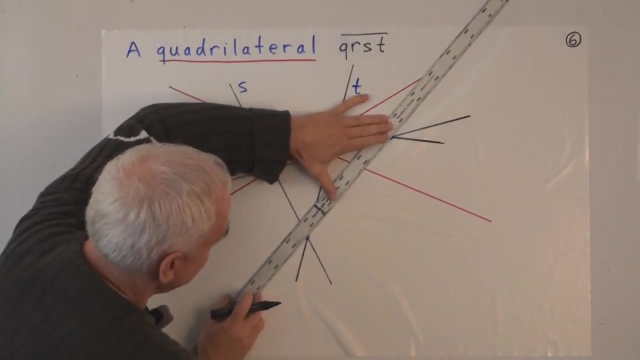 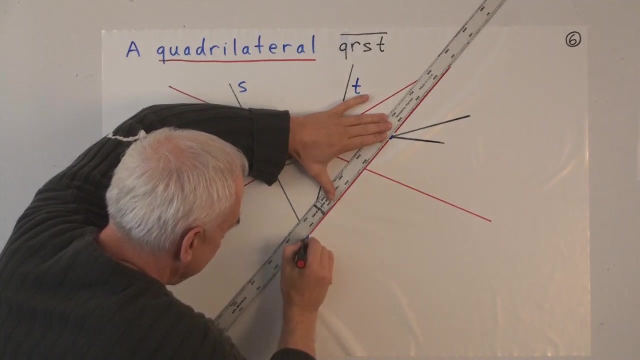 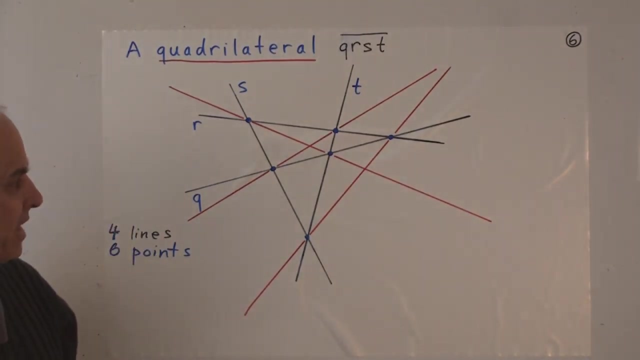 So why don't we join them? Where are some other two points that are not joined? These two points are not joined, Let's join them. And these two points are not joined, Let's join them. Are there any more pairs of blue points which are not joined? 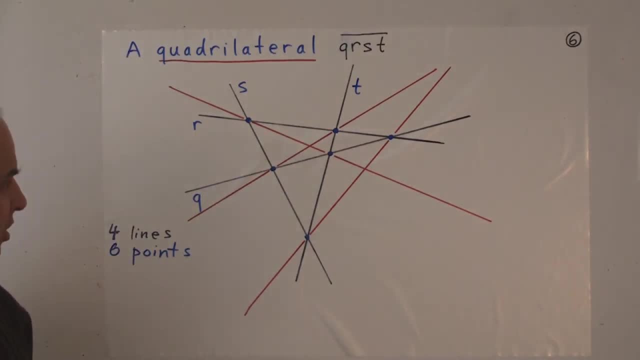 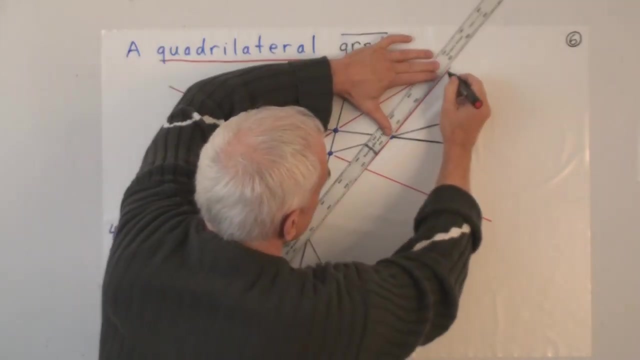 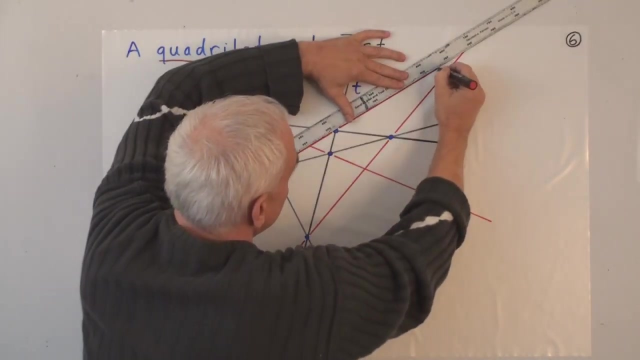 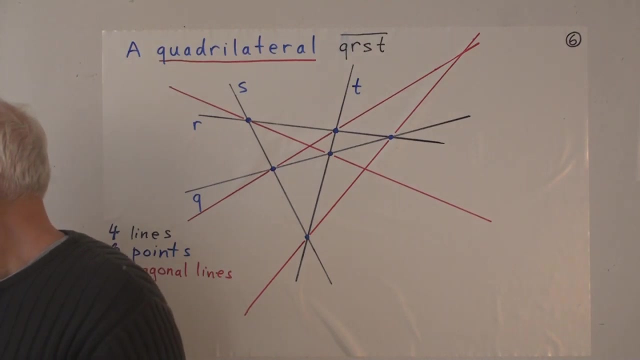 No, We have joined all the blue points And we have now got three diagonal lines In red And I'm going to meet these diagonal lines, Extend them a little bit, Okay, So these three diagonal lines meet in three new points. 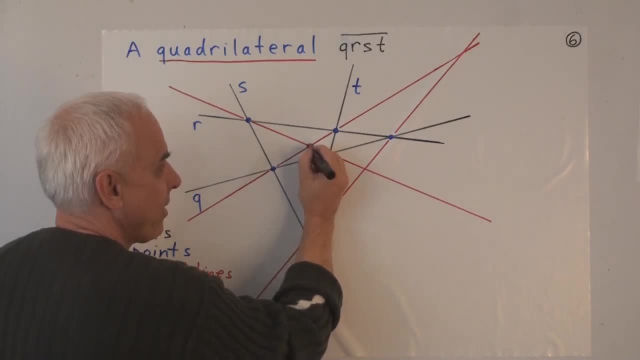 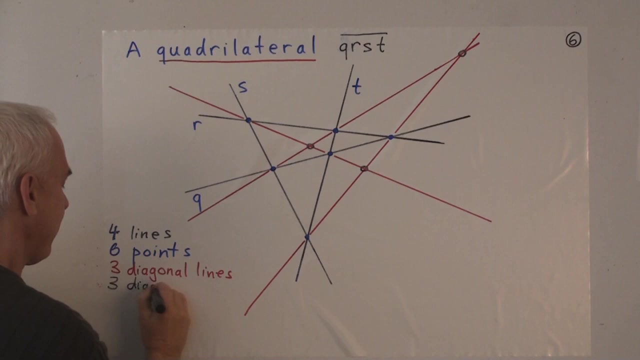 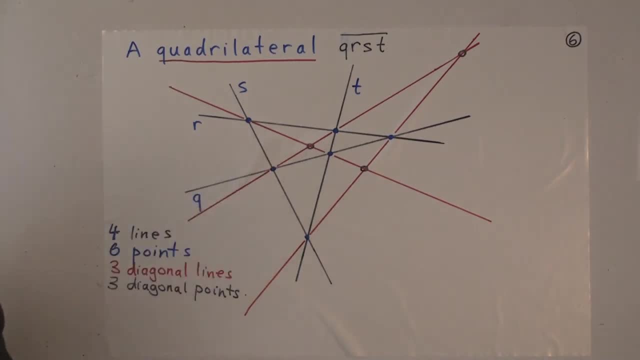 So now, what can we do? All the lines that we have drawn on this page, All the lines that we have drawn on this page, their meets are already recorded, their meets are already recorded. What about the points that we have drawn? Well, a lot of them have been joined. 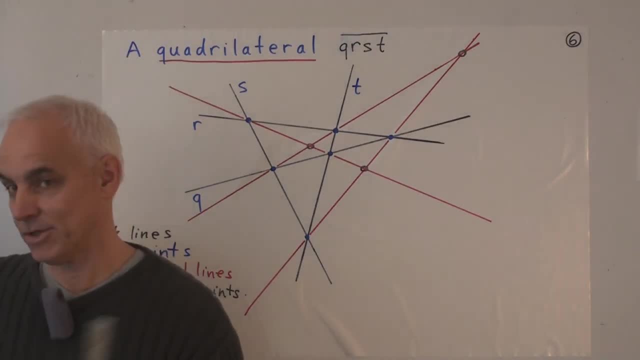 but there are some points which have not yet been joined, So we can join them. Which points have not been joined? Well, this one and this one, for example, haven't been joined. Well, this one and this one, for example, haven't been joined. 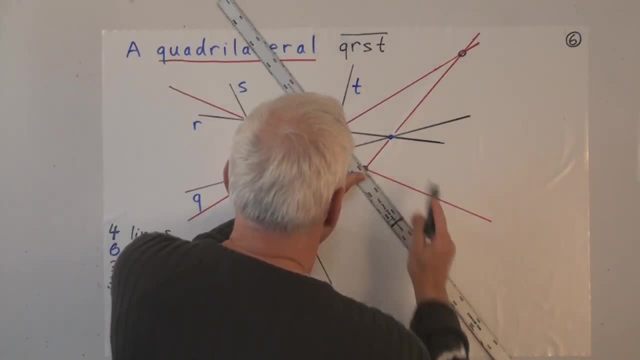 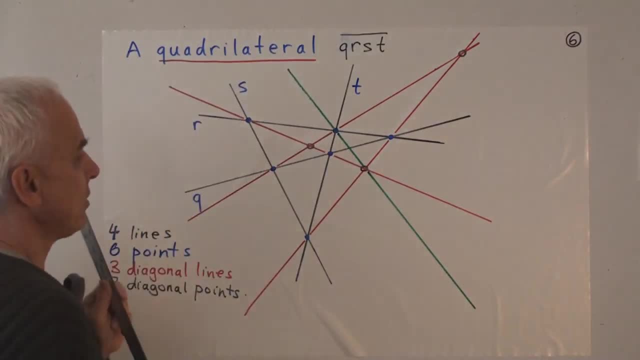 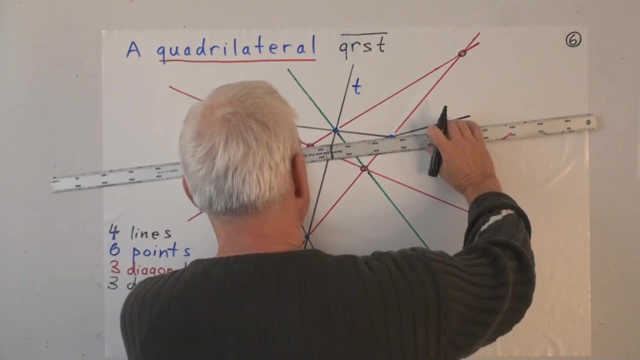 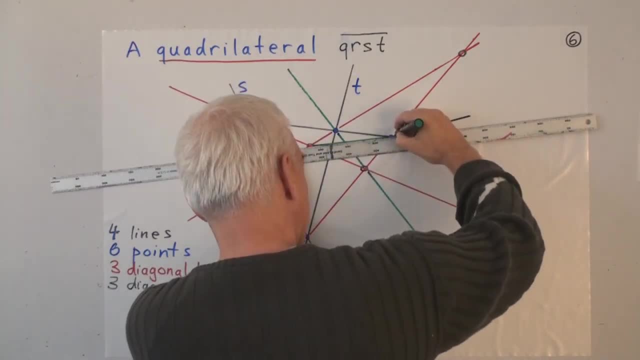 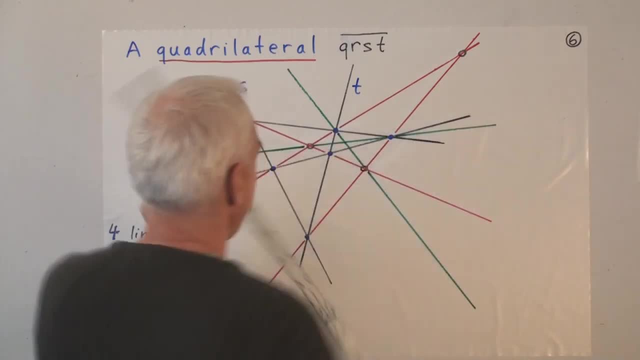 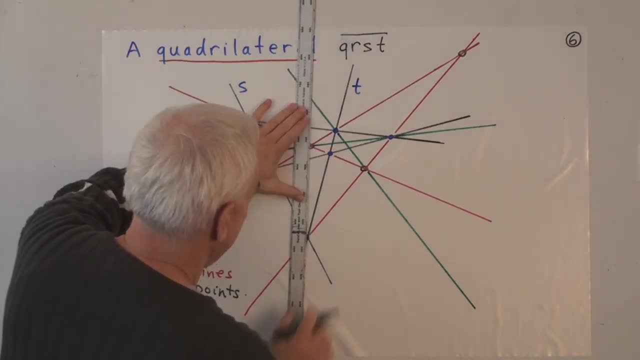 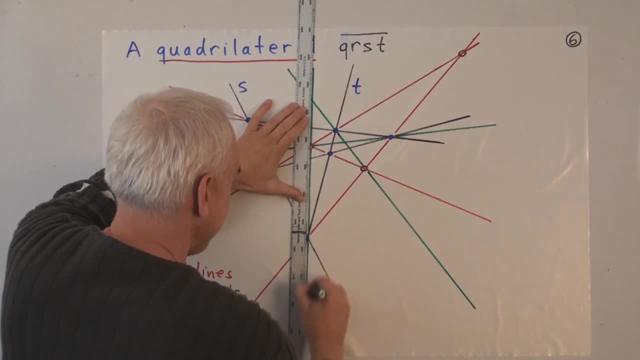 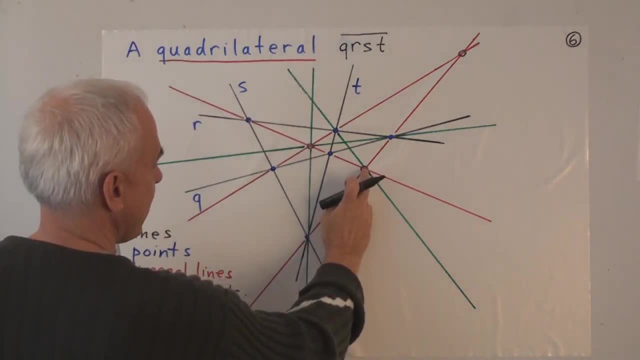 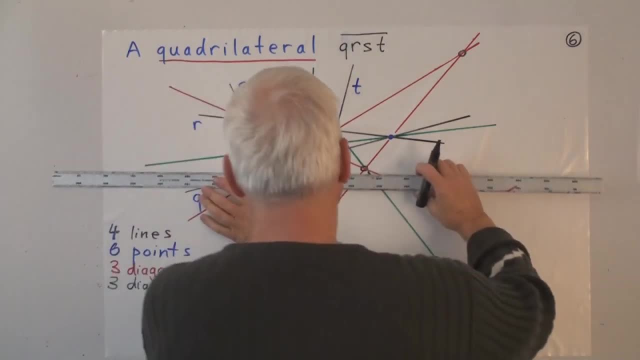 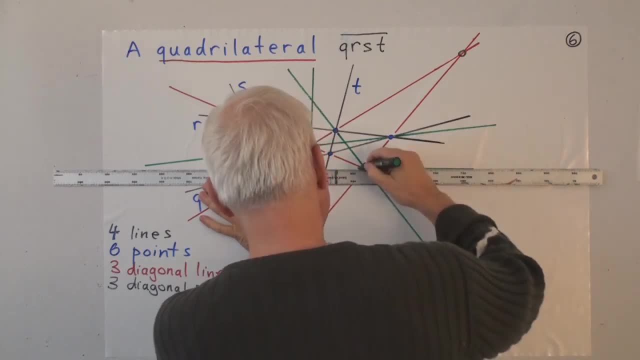 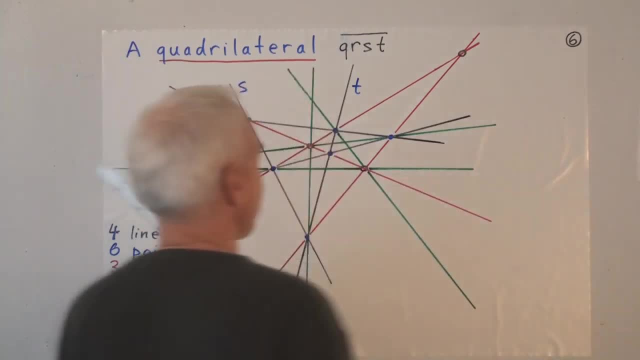 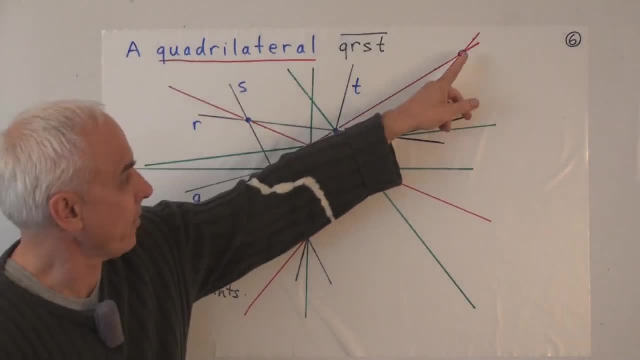 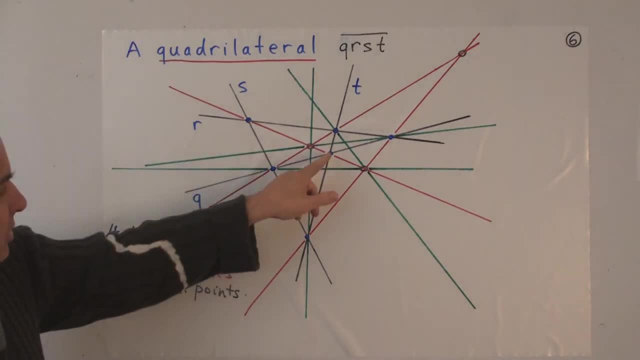 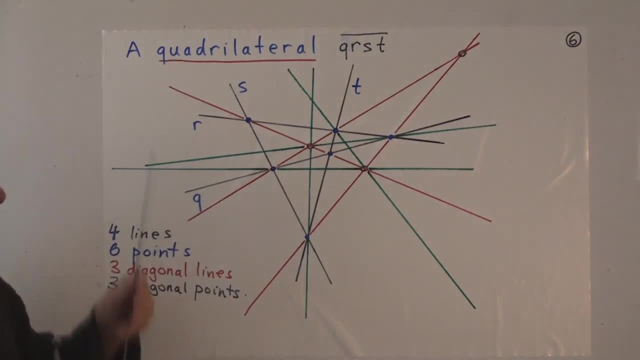 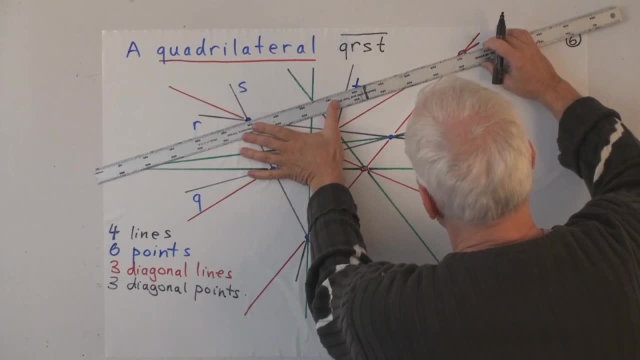 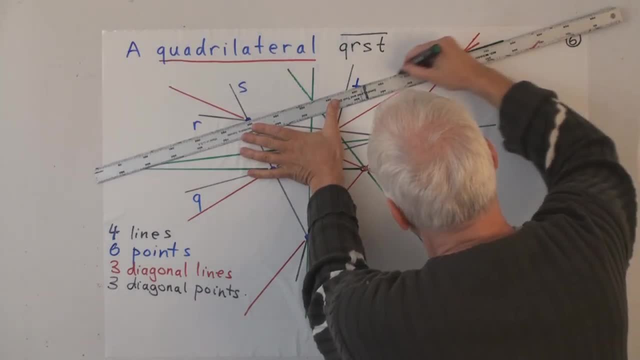 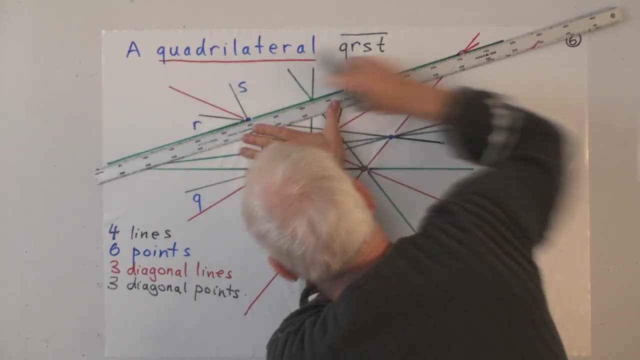 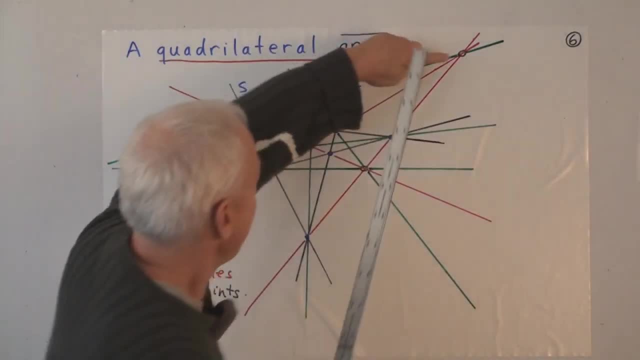 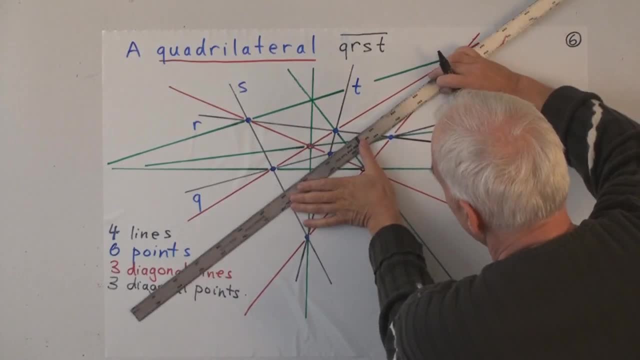 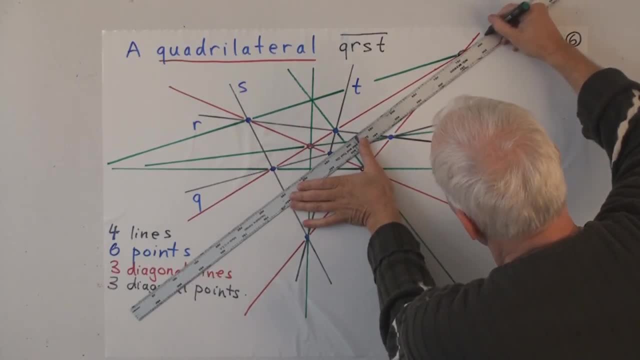 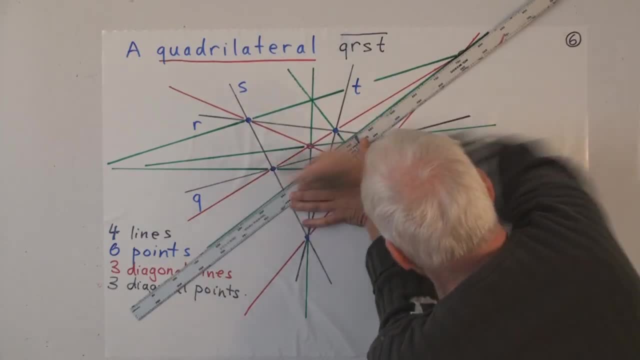 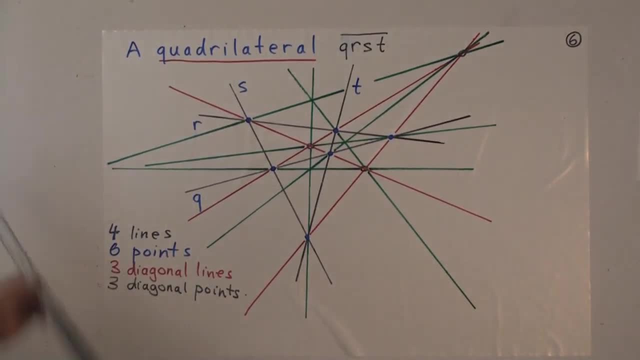 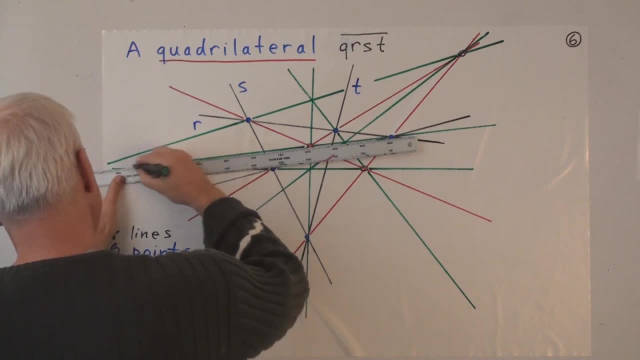 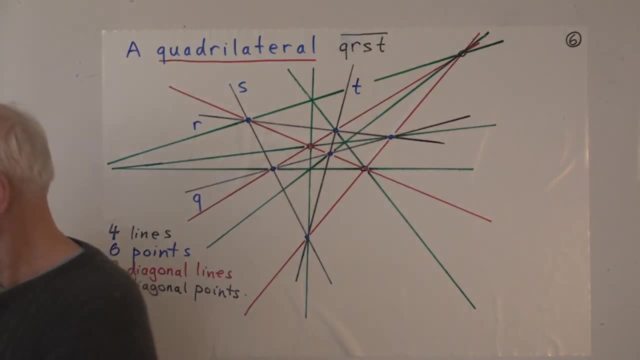 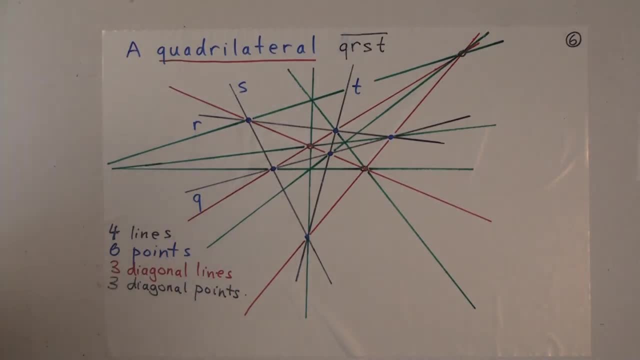 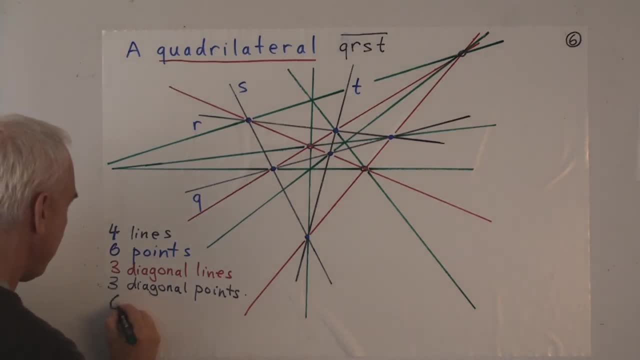 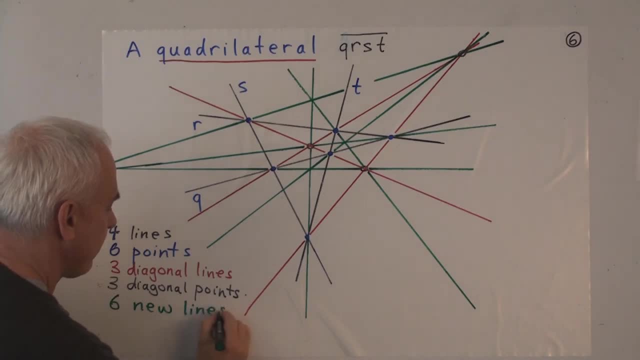 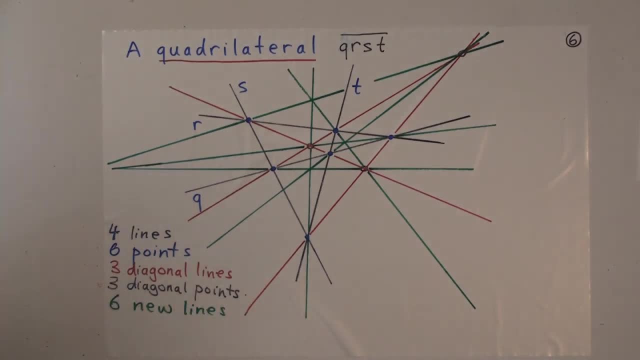 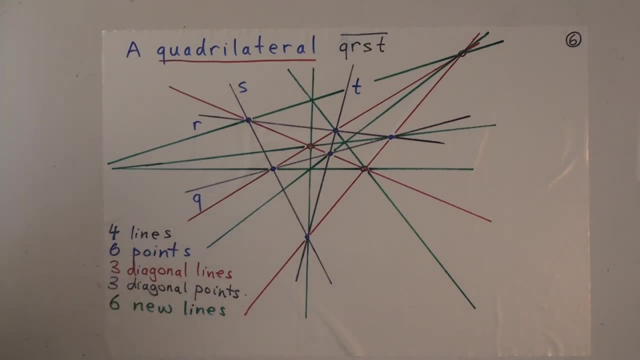 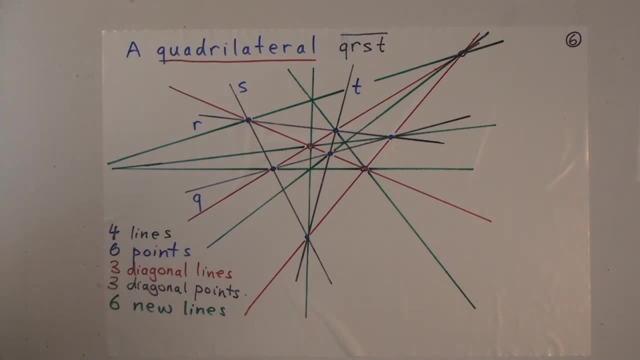 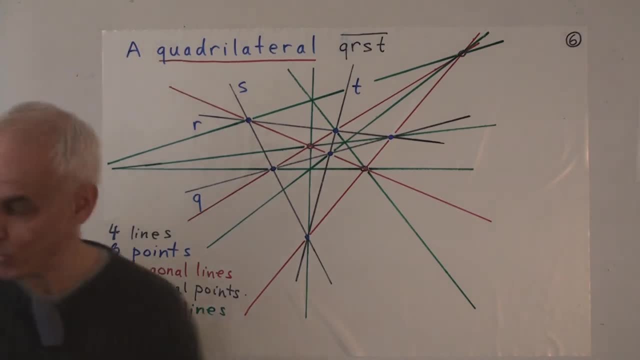 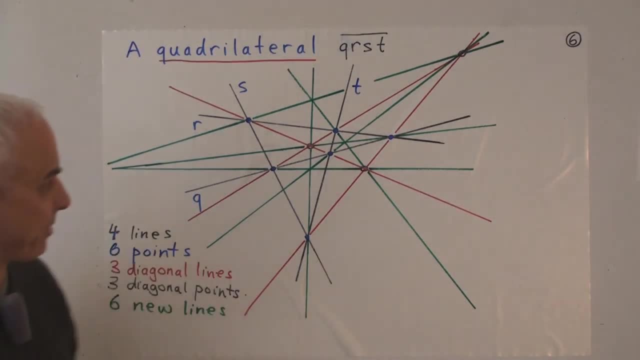 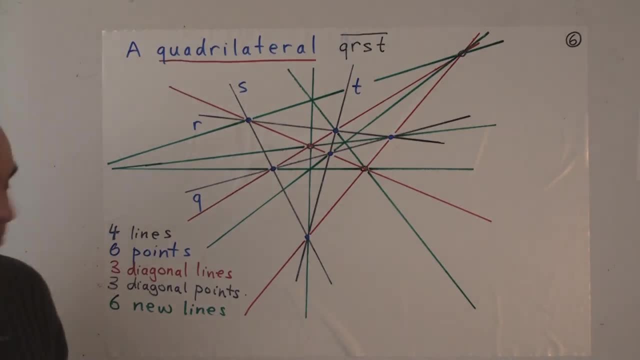 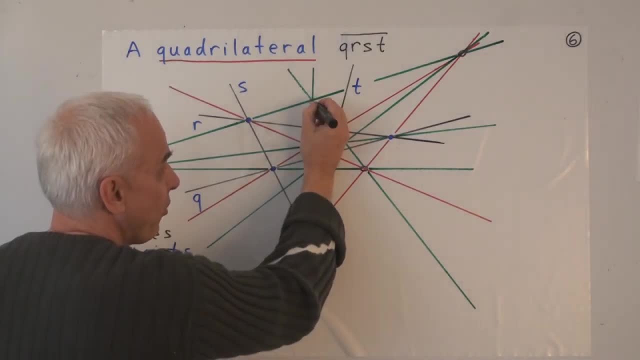 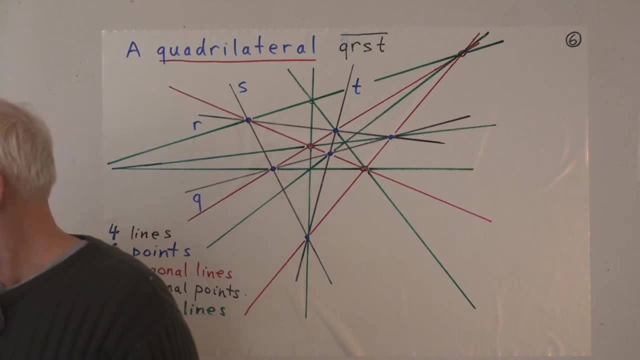 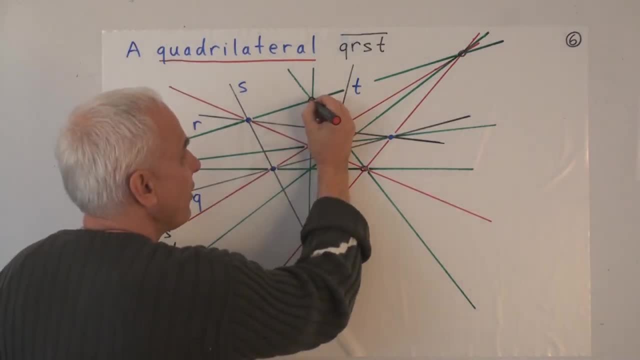 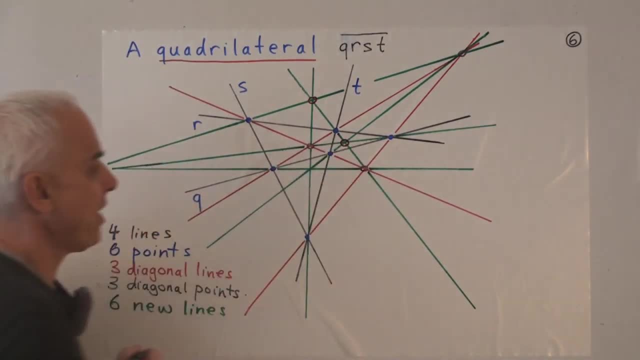 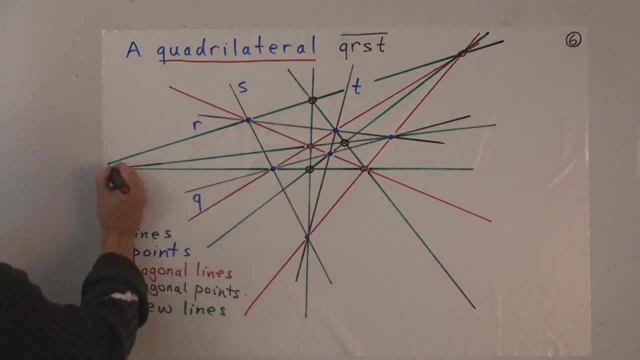 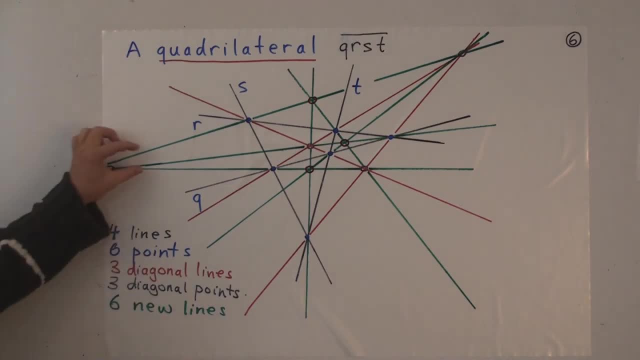 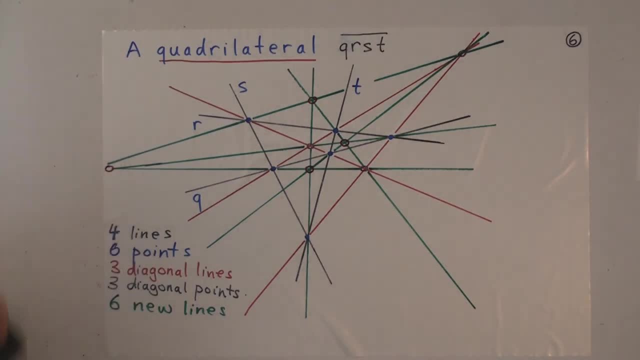 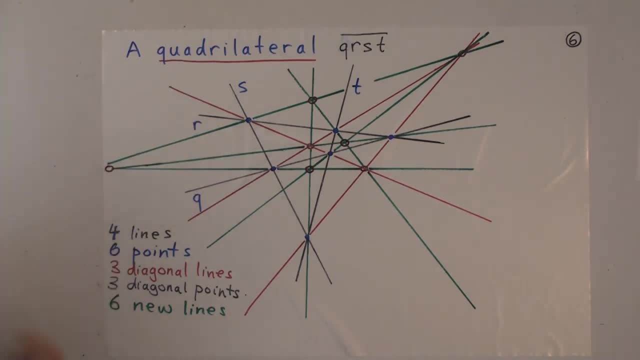 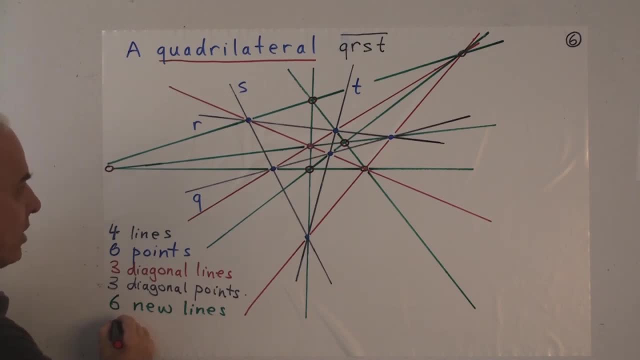 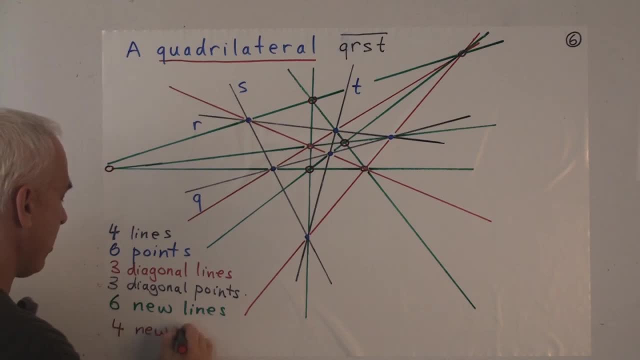 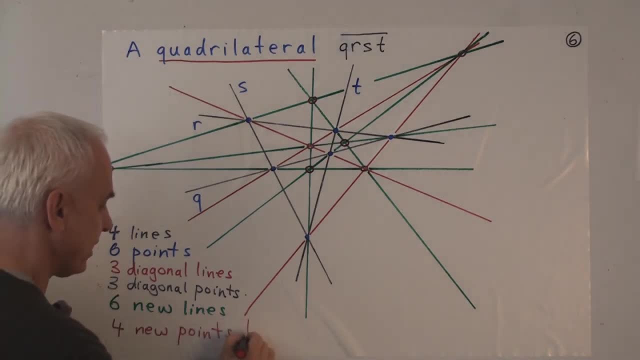 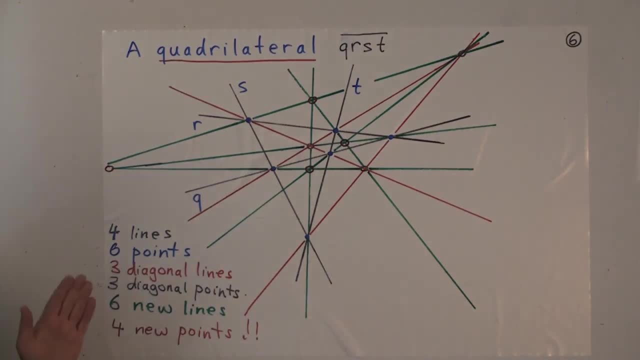 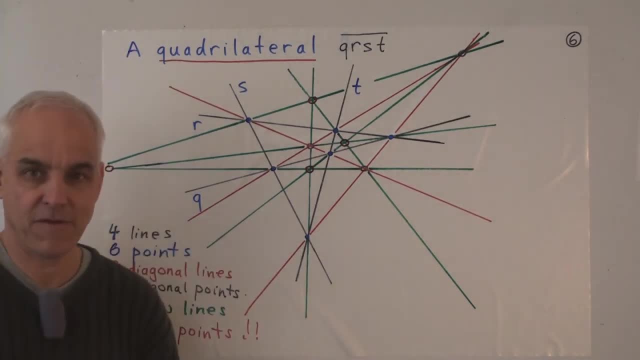 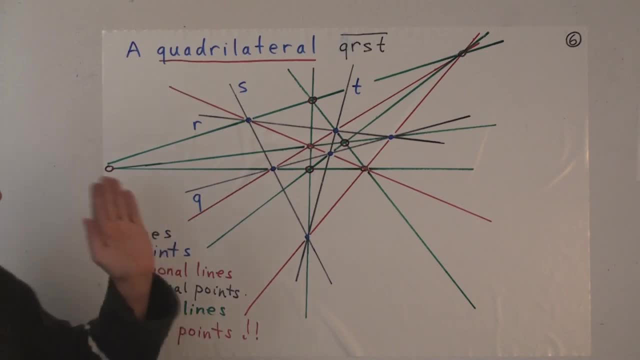 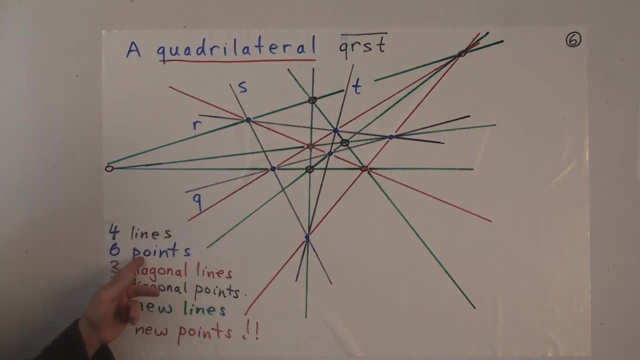 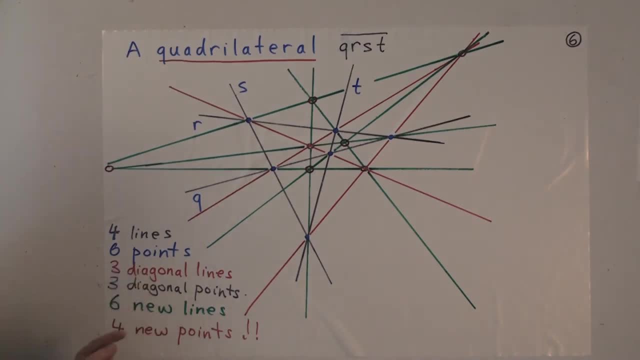 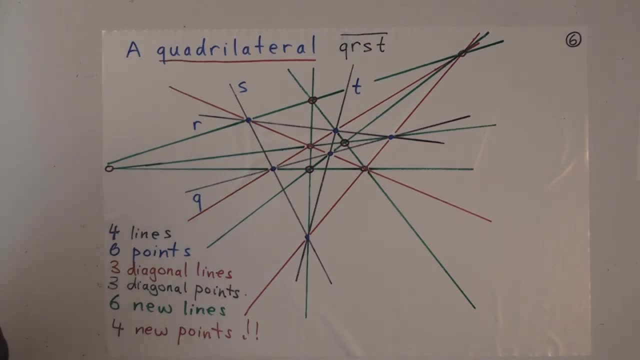 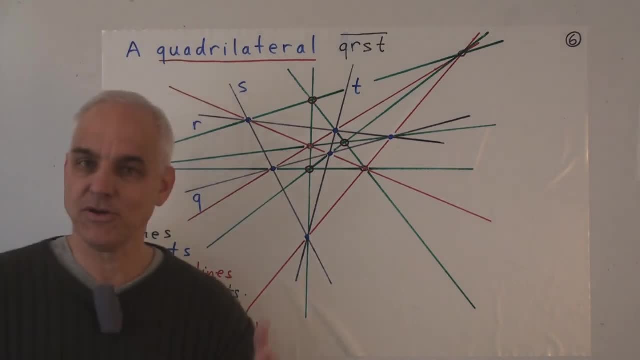 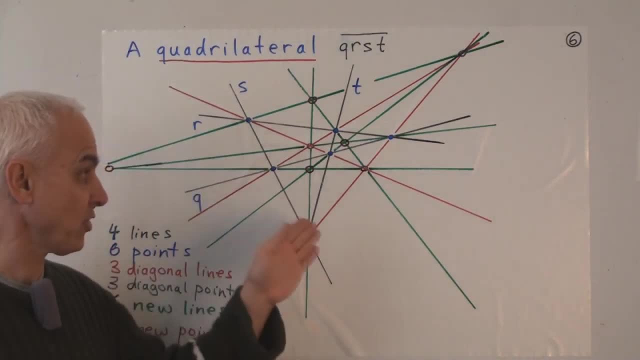 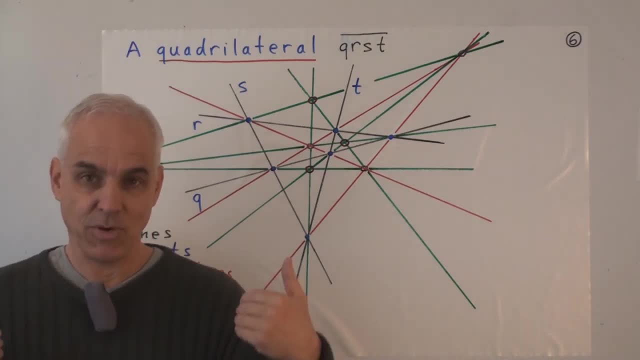 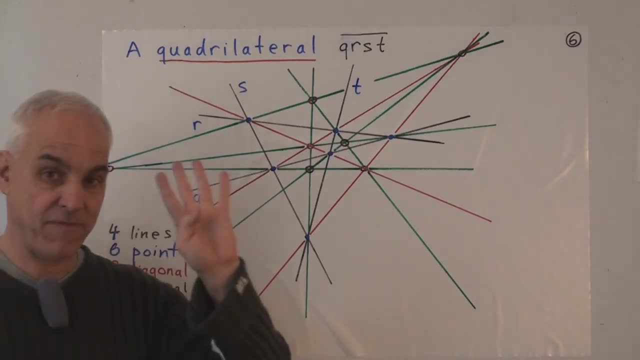 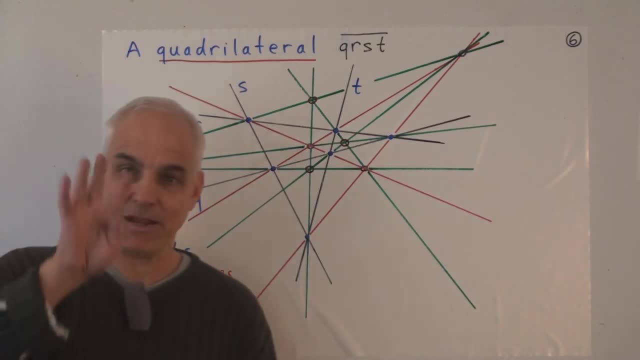 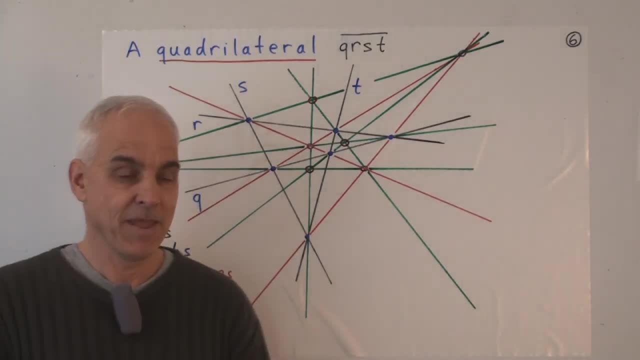 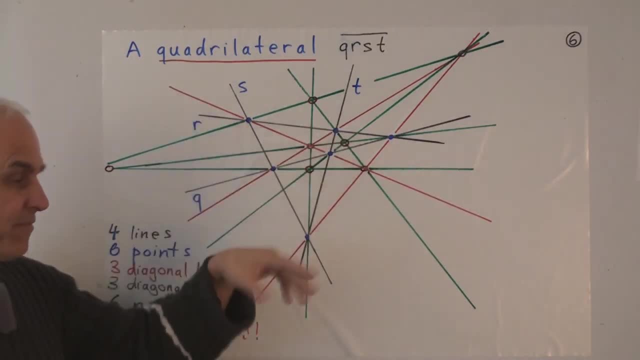 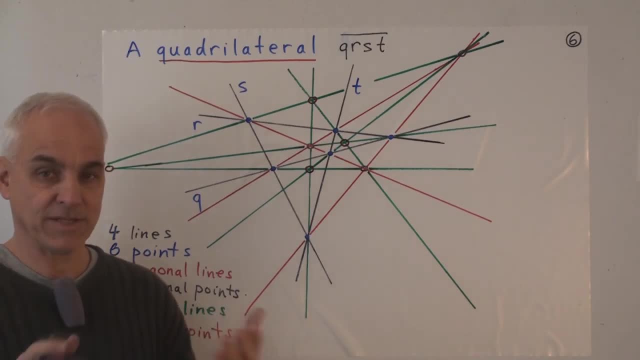 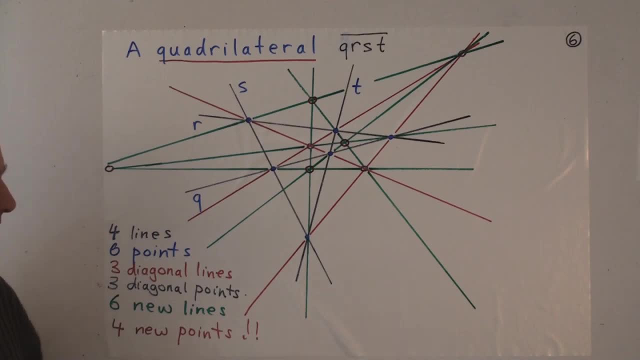 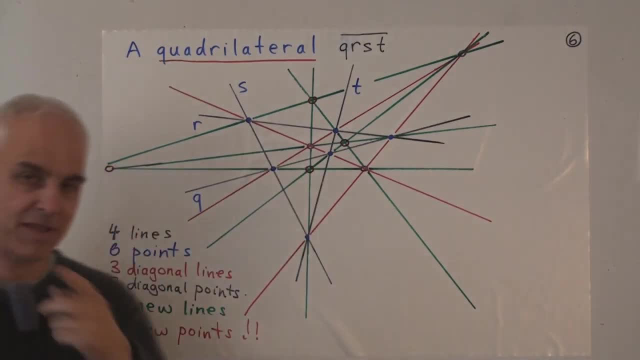 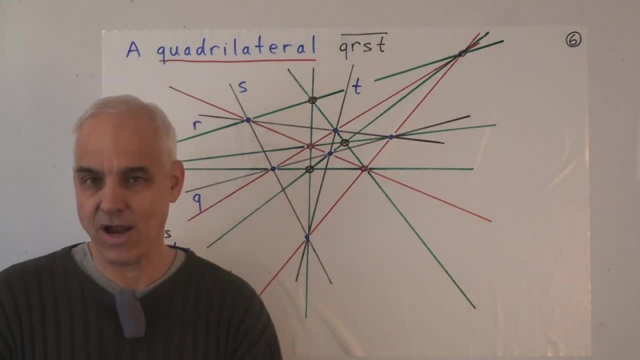 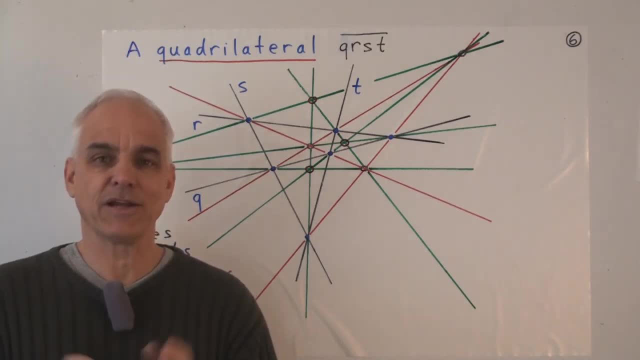 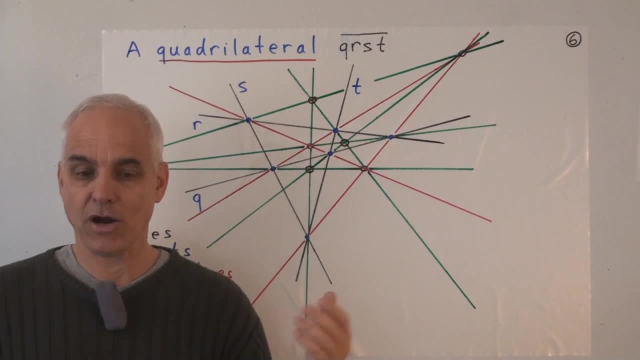 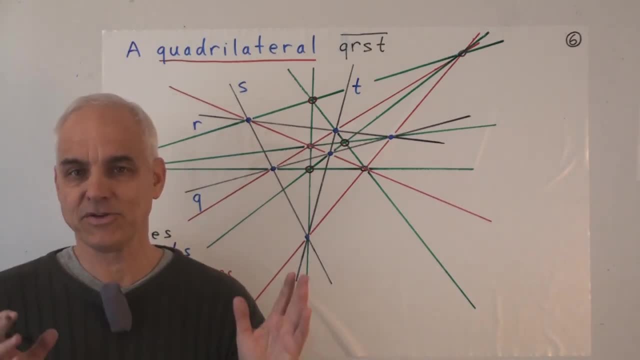 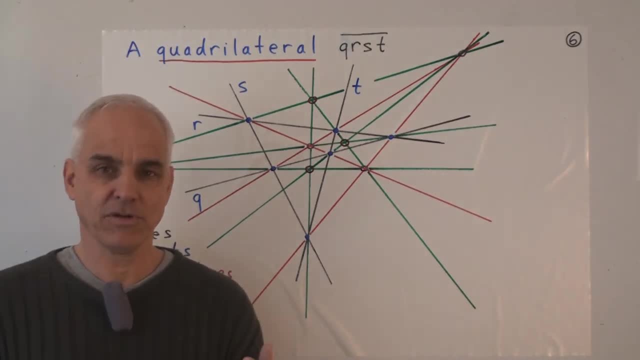 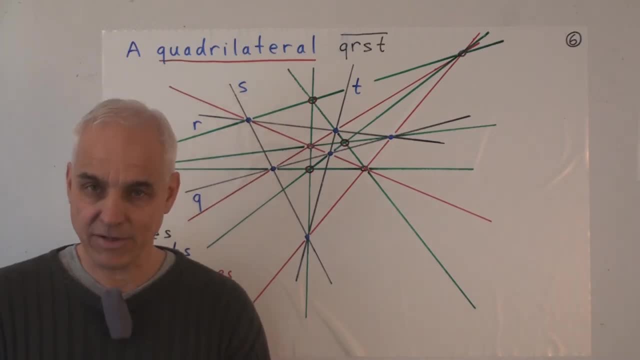 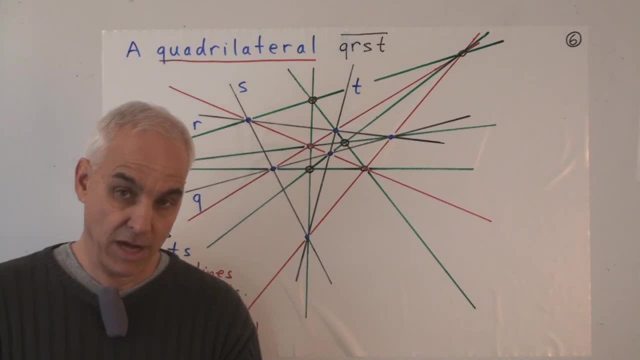 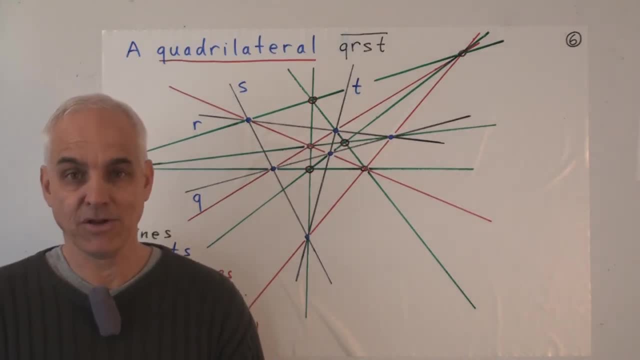 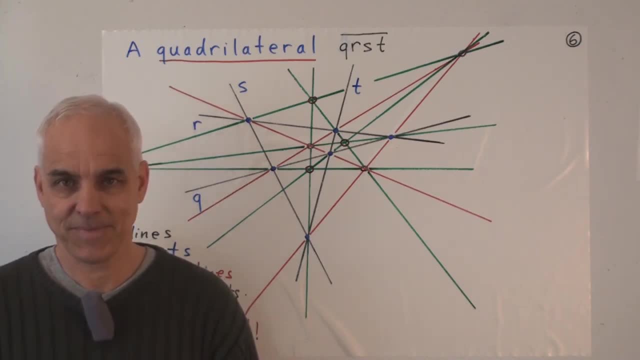 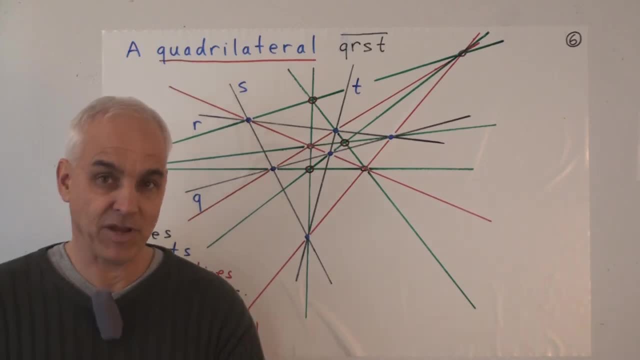 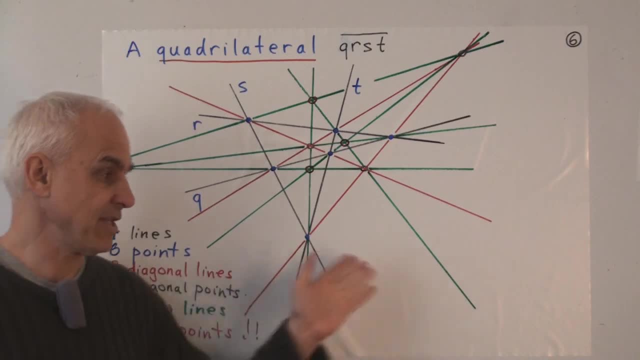 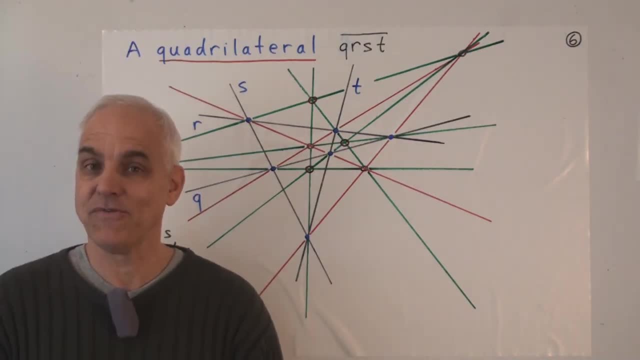 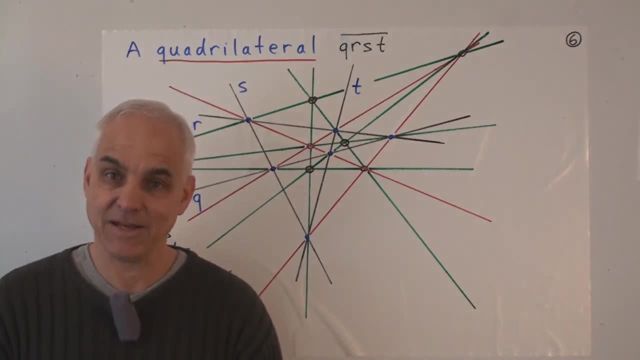 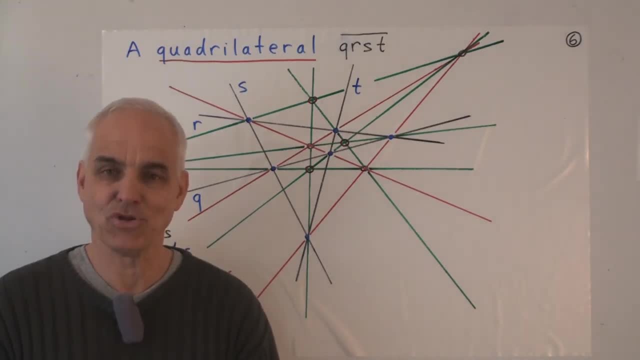